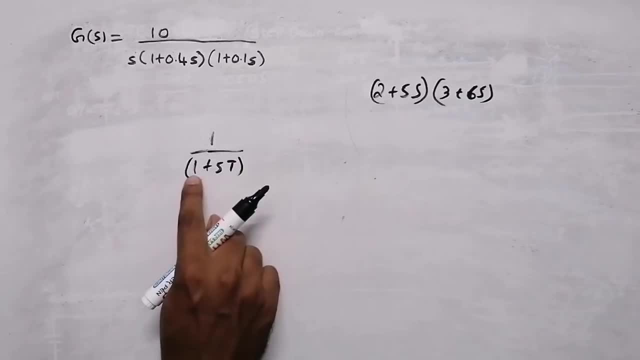 was like this. then is this in a standard form? No, it is not in standard form, So we are going to convert it into 1 plus st. Nearest the value is time. constant. Nearest the value is time. 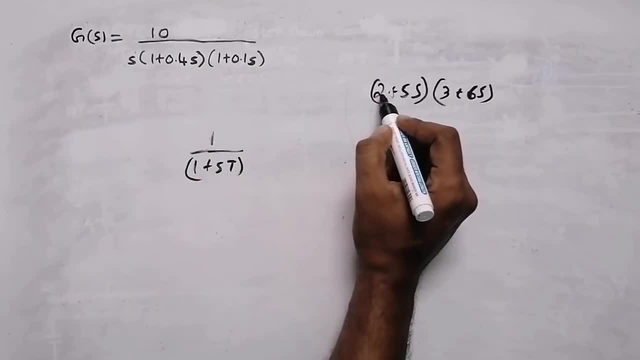 constant, But here the value is not 1. We need to make it as 1.. So for that, what we will do, we will take this 2 outside, Then it will become 1 plus 5 by 2s, And from here we will take 3. 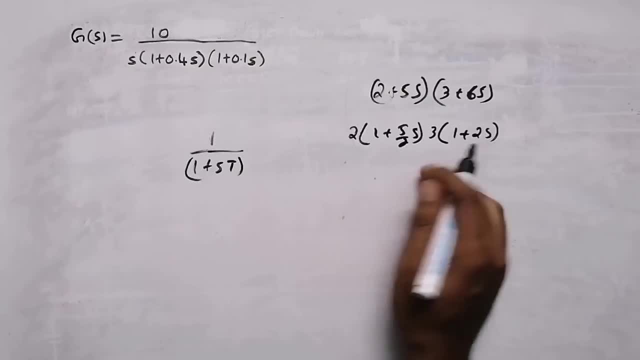 outside And it will become 1 plus 6 by 3. It will be 2, 2s. So this will be the standard form: 1 plus format like this. So in this question it is already in standard form. So we don't want. 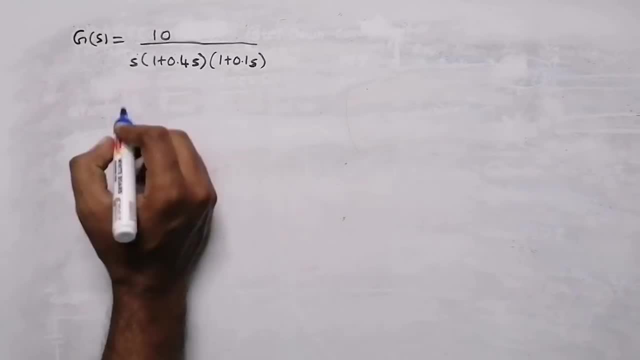 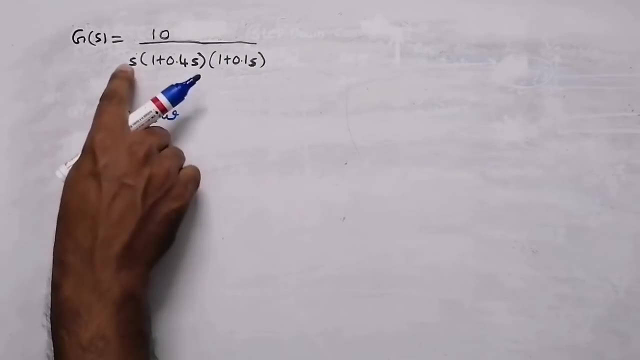 to do anything After making the question in standard form. put sc equal to j omega, because we are drawing the plot in frequency domain, omega frequency. So wherever there is s, you need to replace s with j omega. So here there is s, here all s, here s All those s we need. 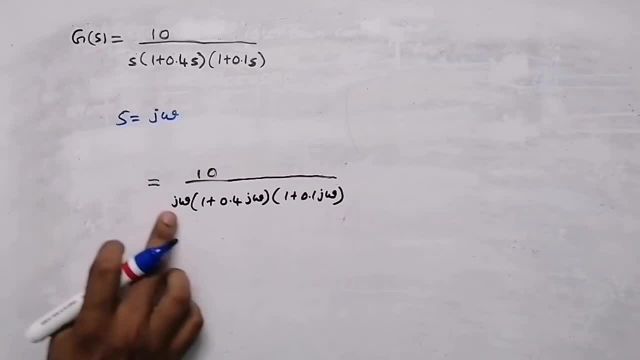 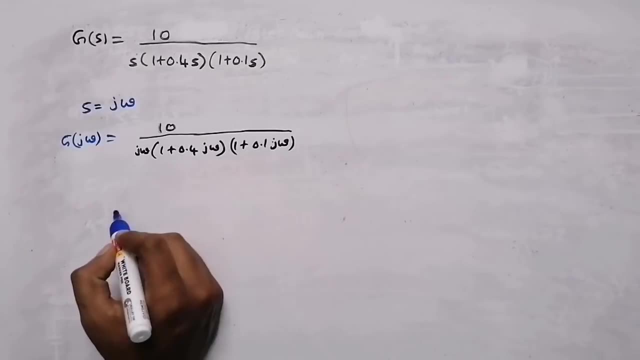 to replace with j omega. So this was our g of s. This is g of j omega. Instead of s, we replaced with j omega. After converting into g of j omega term, we need to plot the magnitude plot We are. 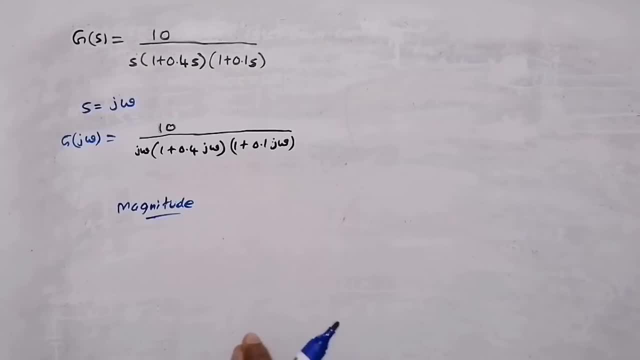 going to draw the magnitude plot. For that we need to find corner frequency. What is going to be corner frequency? Our standard form is 1 plus st, like this. So corner frequency: the value near s it is t Frequency, it is omega. What is the relation between omega and t? 2 pi by t. So 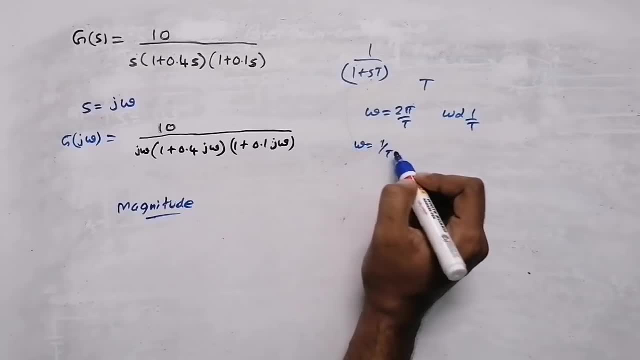 omega is inversely proportional to t, So omega is inversely proportional to t, So omega is inversely proportional to t. So we can write omega equal to 1 by t. The value near s is t, So omega will. 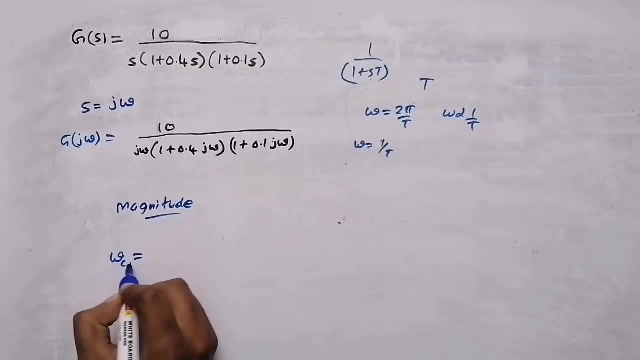 be inversely proportional to that. So first of all we can write our omega c1, corner frequency 1.. The value near s: the value near s. it is 0.4.. Inverse of that: 1 by 0.4.. What is that? 2.5. 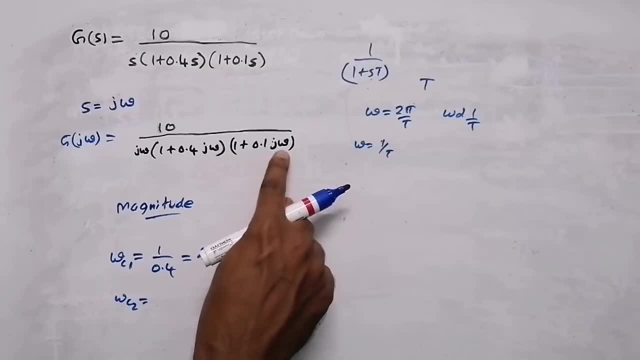 radian per second. Now the second corner: frequency. the value near s. the value near s it is 0.1.. So inverse of that, 1 by 0.1. It is 10, 10 radian per second. So these two are the corner. 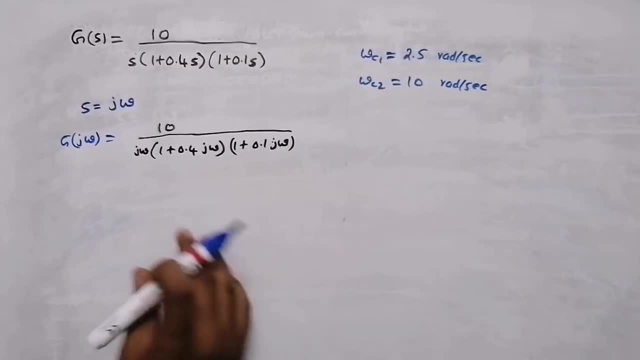 frequencies. After finding the corner frequencies, we need to check the number of terms in this equation. So there are three terms. One is 10 by j omega. that is our first term. Then 1 by 1 plus 0.4, 1 plus 0.4 j omega, that is our. 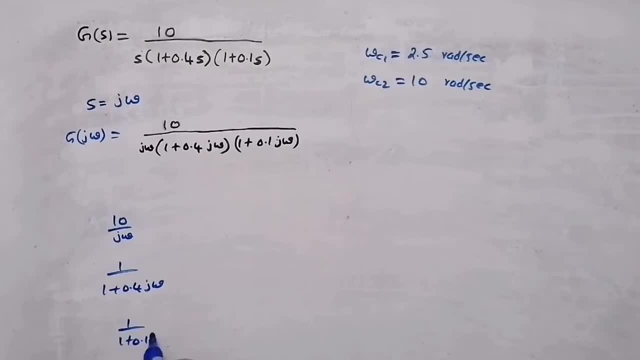 second term, And this is the third term, 1 by 1 plus 0.1 j omega. So these are our terms. We have three terms in this equation. Now we are going to draw a table, okay, First, 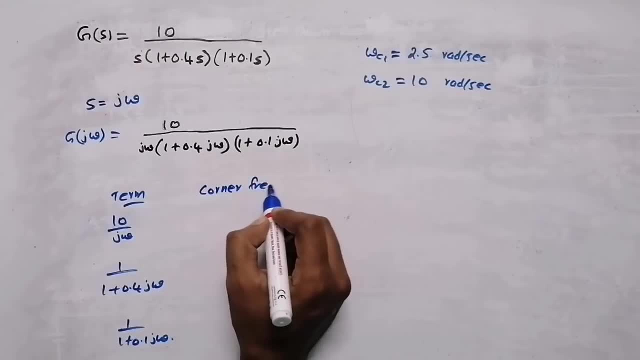 of all, write the terms, Then write the corner frequency, Then write the slope, Then write the change in slope. So we need to draw a table like this. So the first term it is 10 by j omega. What will be the corner frequency? There is no. 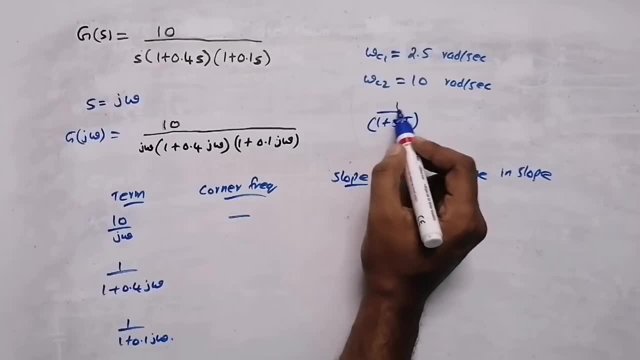 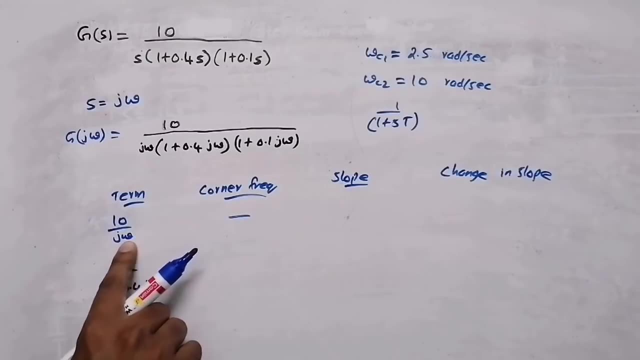 corner frequency, because you need to get that in a standard form like this: 1 by 1 plus 60. Here it is. only s, is there? We need it in the standard form like this: okay, So there are no corner frequency. Then slope- How to find slope If s, that is our j omega is? 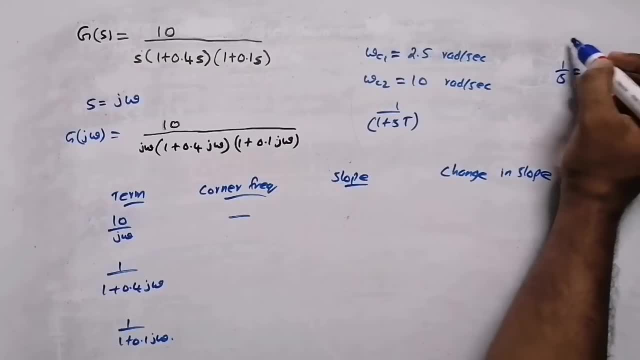 in the denominator. If s is in the denominator, the slope will be minus 20.. If s is in the numerator, the slope will be plus 20.. If it is s square, the slope will be plus 40.. If it is s cube, the slope will be plus 60.. If s square is in the denominator, the slope 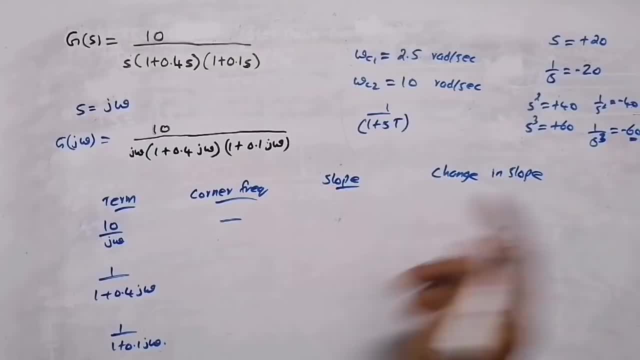 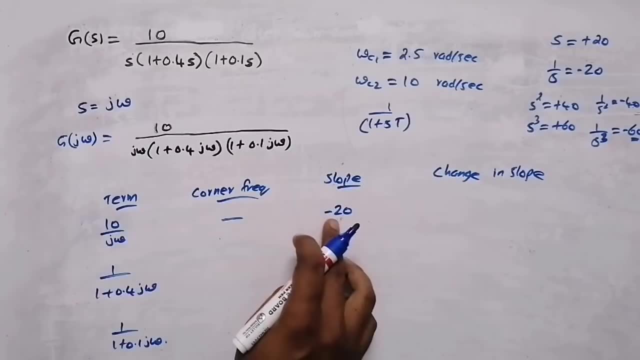 will be minus 60, like this. So in this term the s or j omega term is in the denominator, So the slope will be minus 20.. In the denominator the slope will be minus, In the numerator the slope will be plus. And when square comes 40. Cube comes 60. Then s raise to 4, the 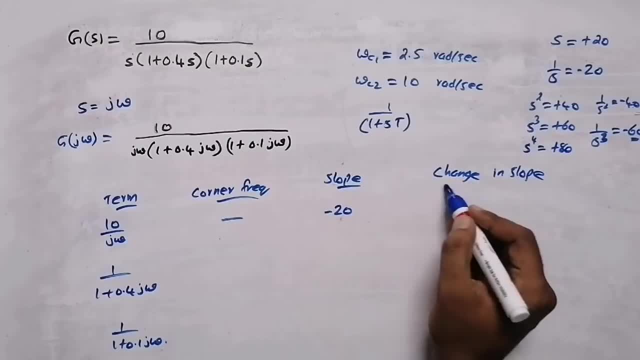 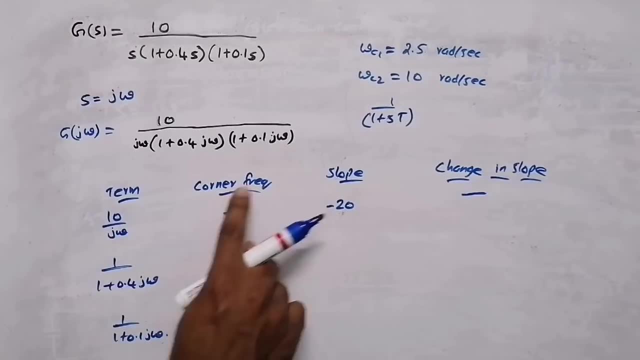 slope will be plus 80, like that It will go okay. So slope is minus 20.. Then the change in slope. Is there a change in slope? No, We are starting only So there is no change in slope. Now the second term. Second term: the corner frequency: we already found. 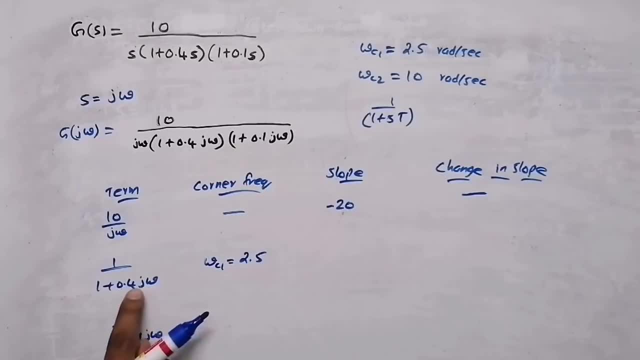 it is 2.5.. That is of omega c1, it is 2.5.. The value near s it is 0.5.. So it is 2.5.. The value near s it is 0.4.. Inverse of that we need to take: So that is 2.5.. And the 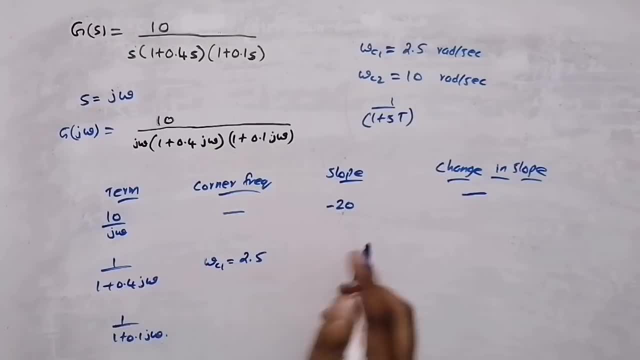 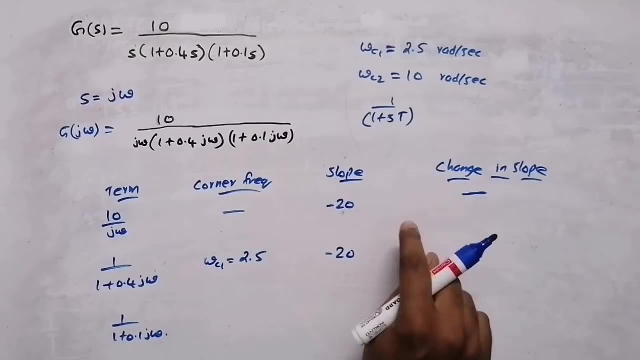 slope. Here the denominator, the power, is s. It is in the denominator, So it will be minus 20.. If it was j omega square, the slope will be minus 40. But here it is minus j omega, So the slope is minus 20.. Now, change in slope. Now there is a change in slope. 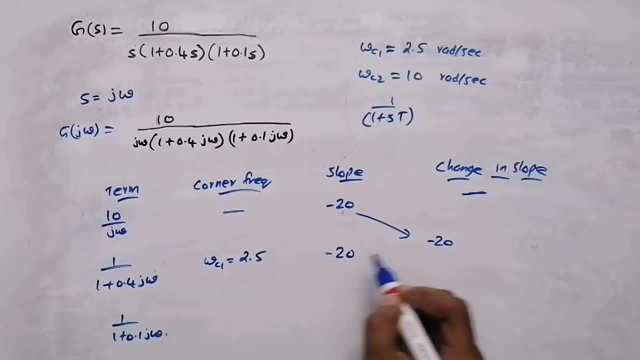 For minus 20, it becomes minus 20.. So minus 20 was our initial slope. Then again a minus 20 slope is getting, Minus 20 slope is getting So minus 20, minus 20, it will be minus 40.. 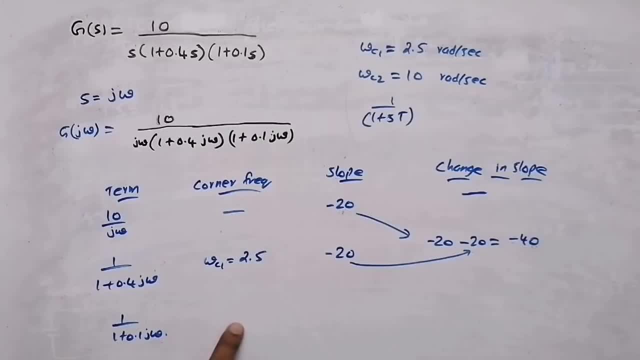 That is our change in slope. Now the third term. Third term: corner frequency. we already found it is 10 radian per second. It is our omega c2.. Corner frequency is 10 radian per second. The value near s it is. 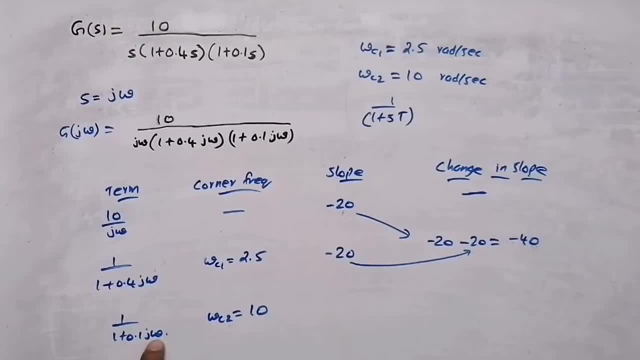 0.1.. Inverse of that, we will get 10.. Now slope: The s term is in the denominator And it is already s. It is not s square or s cube, It is s. So the slope will be minus 20 because 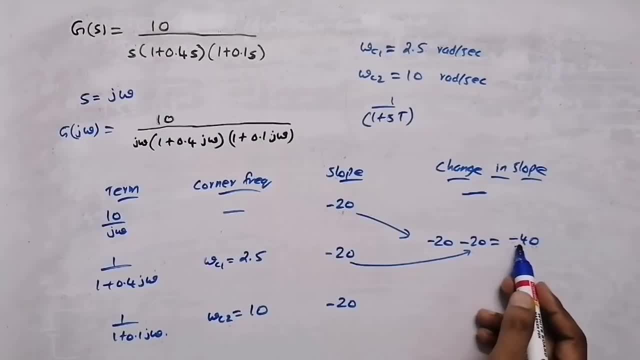 it is in the denominator. Now, change in slope. The slope was minus 40. The previous slope was minus 40. Then a new slope of minus 20 is coming. So minus 40, minus 20, it will be minus 60. That is the change in slope. Before finding the slope and change in slope: 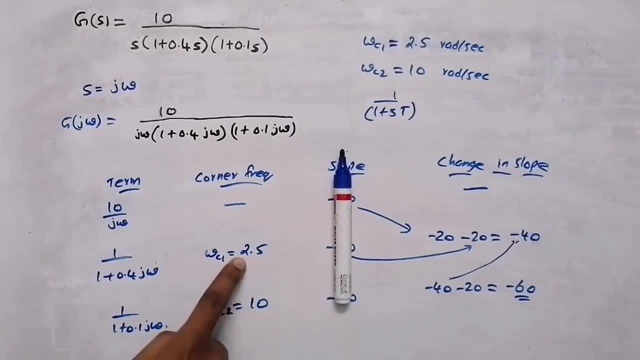 after writing corner frequency: you need to check whether the corner frequency is in ascending order. So here it is in ascending order, There is no problem. So here it is in ascending order, There is no problem. First you need to check whether the corner frequency is in ascending order, Then only 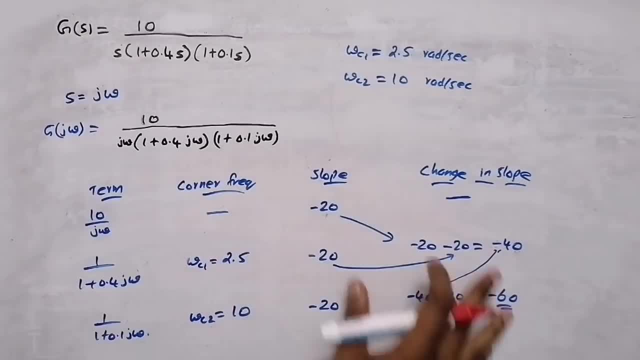 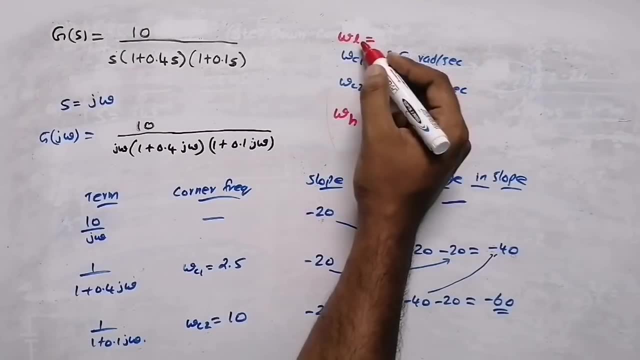 you need to find slope and change in slope. Now, after drawing the table containing corner, frequency, slope, change in slope, you need to select two frequencies, That is, omega- lower frequency and omega- higher frequency. You need to select two frequencies: Omega. 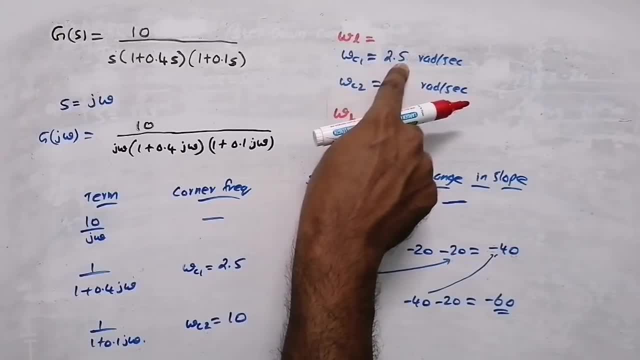 lower should be less than our first corner frequency. So here it is 2.5.. So omega lower should be less than 2.5.. You can select 2.. You can select 0.5.. You should not select. 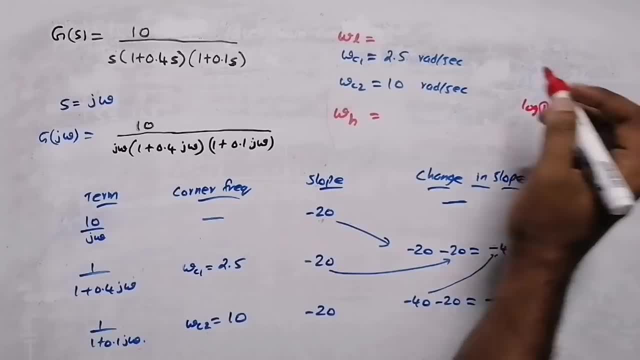 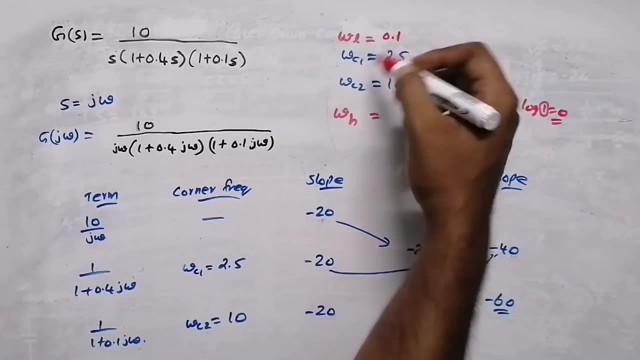 1 because log 1 is 0. So you do not select 1 as the lower corner frequency Other than 1, any value less than our first corner frequency we can take. I usually take 0.1 as my lower corner frequency. You can take any value Less than 2.5, any. 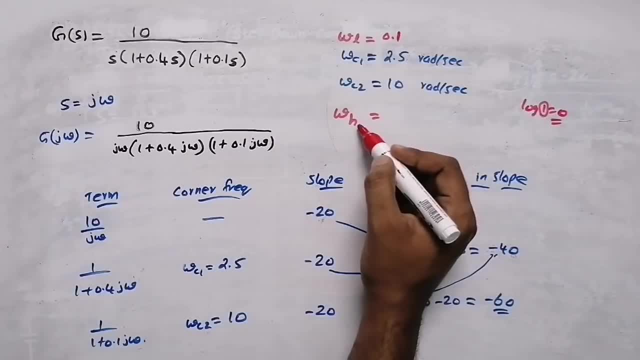 value you can take. I used to take 0.1 as my lower frequency, Then omega higher. Omega higher should be greater than omega c2.. Omega c2 is 10.. So you can take any values greater than that: 20,, 30,, 40,, 50,, 100, anything. I am taking it as 100.. Okay, So this is my 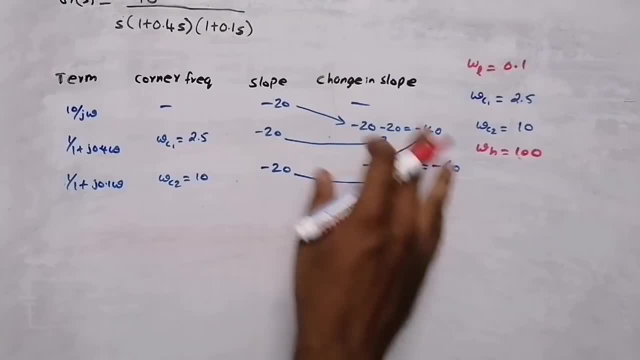 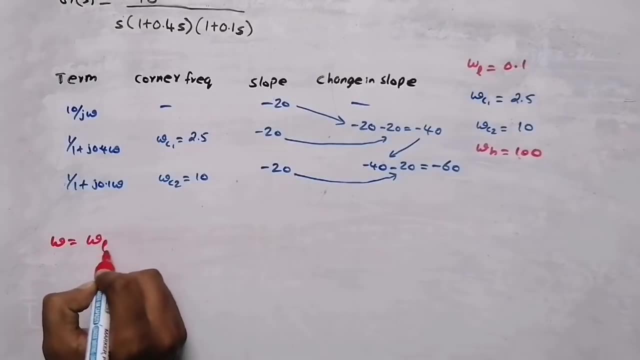 omega lower and this is my omega higher. From this table and also from this frequency, we are going to find the magnitude. So, first of all, we can find the magnitude when omega equal to omega lower. When omega equal to omega lower, what will be our magnitude? 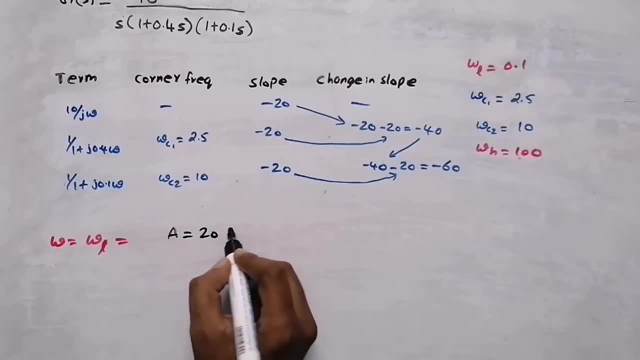 For finding magnitude. the equation is: A is our magnitude. The equation is 20 log first term. What is our first term? 10 by j omega. 10 by j omega. It is magnitude. we need to take, Okay, 20 log 10 divided by 4 j omega. We need to substitute the value for: 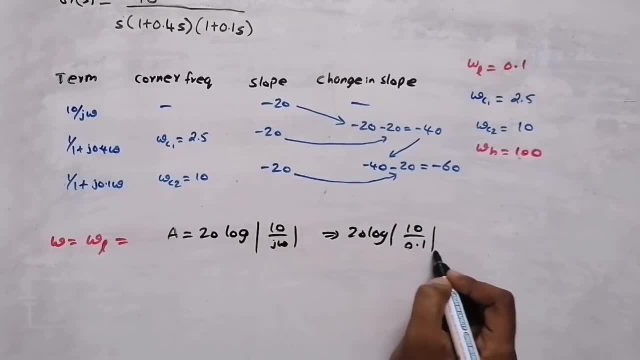 omega. Omega is 0.1.. That is our lower value. So 10 by 0.1.. So when we solve in calculator we will get the answer as 40 dB. That is our first magnitude when omega equal to omega. 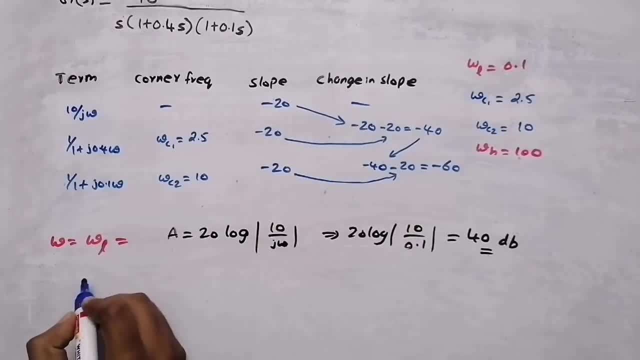 lower. Now we need to take the next frequency, omega c1.. When omega equal to omega c1. So our first corner, frequency. In these two terms the equation will be same. That is the equation for magnitude. Finding magnitude is same: 10 divided by j omega. So we can 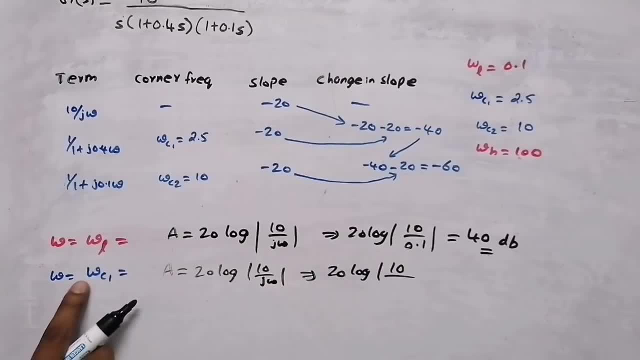 substitute it: 20 log 10 divided by 4 j. omega, We need to substitute the value of omega c1.. Omega c1, the value is 2.5.. So 2.5.. We will get the answer as 12.04.. We can approximate. 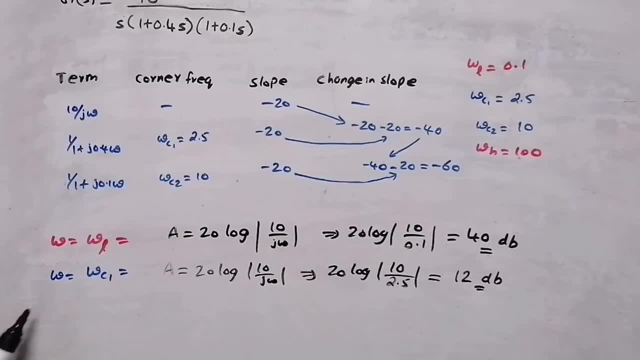 it into 12 dB. That is our second magnitude, when omega equal to omega c1.. Now for omega c2.. From here onwards there will be change in our equation for finding magnitude When omega equal to omega c2.. Second corner frequency: The equation will be for finding the magnitude. 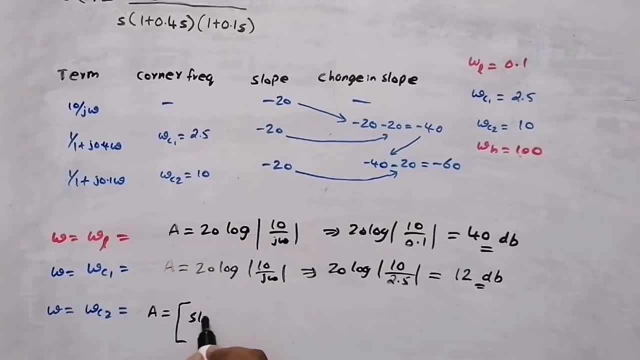 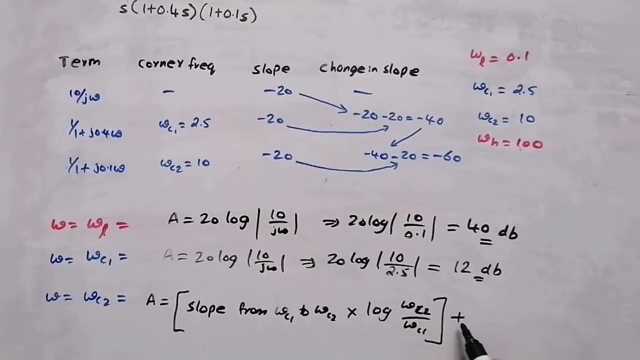 the equation will be a equal to. we need to find the slope. We got slope Slope from the previous value, that is, omega c1. Omega c1 to our value, omega c2, into multiplied by log of omega c2, divided by omega c1 plus magnitude of our previous value, that is, at omega c1.. 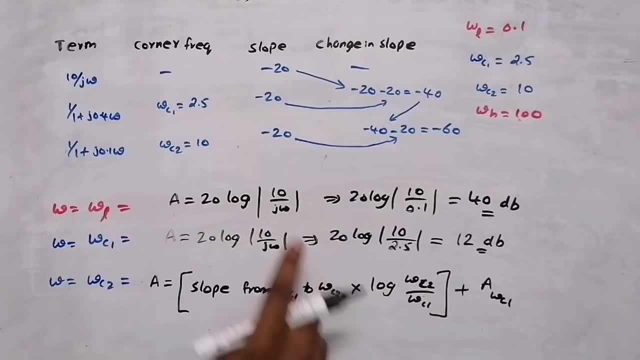 We can substitute that Slope from omega c1 to omega c2.. Omega c1 to omega c2, the slope be minus 40. So we are going to substitute minus 40 multiplied by log omega c2.. Omega c2, the value. 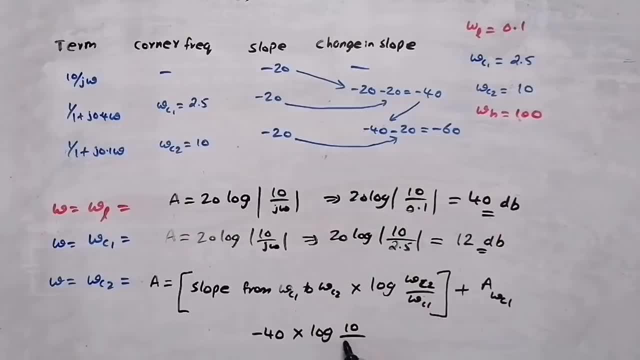 is 10.. Then the previous value, that is, 2.5.. Omega c2 by omega c1. Omega c2 is 10, omega c1 is 2.5.. So that should be added with magnitude when omega c1. At omega c1, the magnitude is 12.. 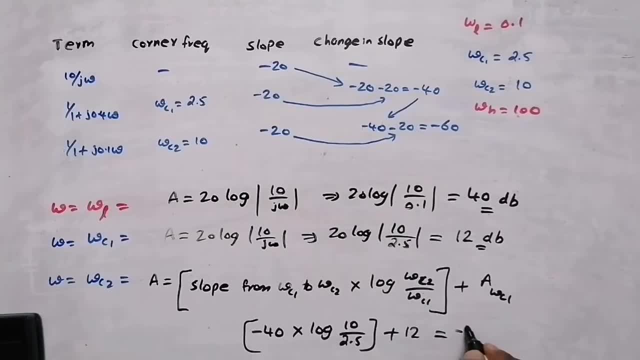 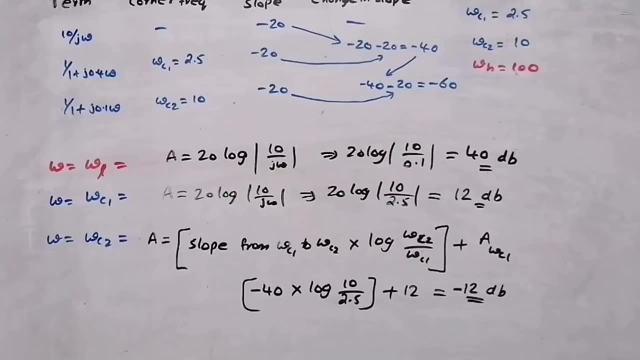 So when we solve this in calculator, you will get minus 12.08,. we can approximate it into minus 12 dB. That is our magnitude when omega c2.. Now for omega higher. we need to find the slope, So we need a magnitude for that omega higher. when omega equal to omega higher. For omega higher also. 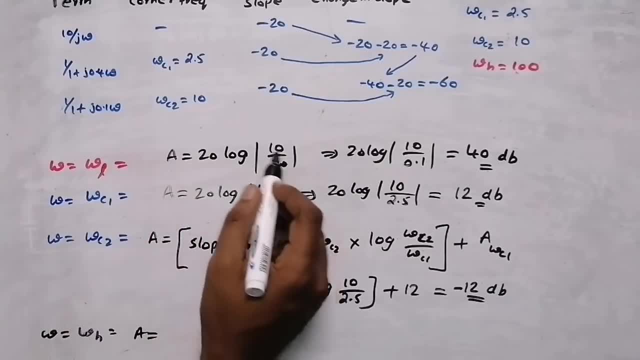 the equation is same Only for the first two omegas. the equation is this thing: 20 log first term. For all other frequencies, the equation will be like this: So slope from where to where, From omega higher to previous value. Omega higher to previous value: it is omega c2.. Omega c2,. 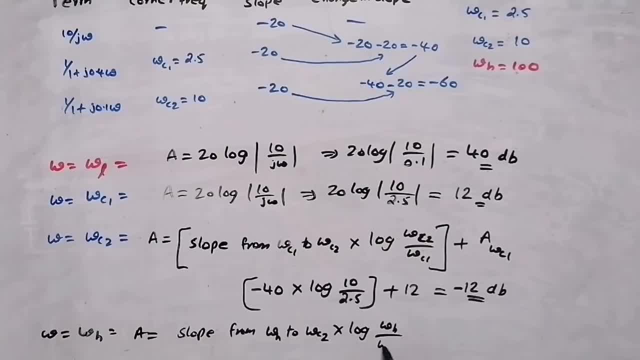 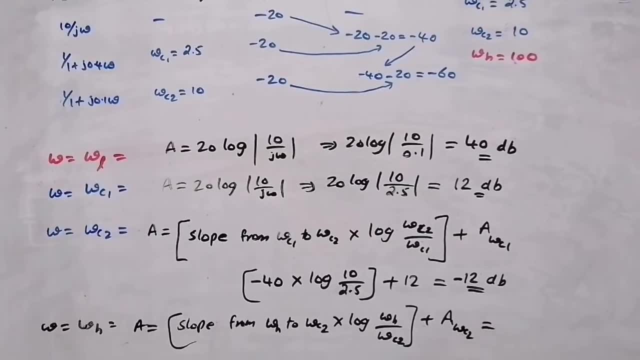 it should be multiplied with log omega higher divided by previous value. That should be added with magnitude of previous value. Previous value: it is omega c2.. So what we will get: Slope from omega higher to omega c2.. Slope: it is minus 60.. Minus 60 should. 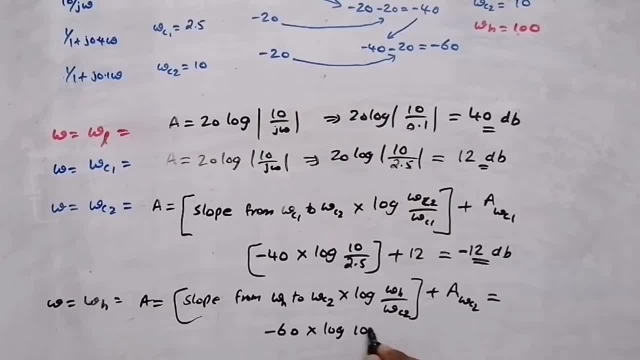 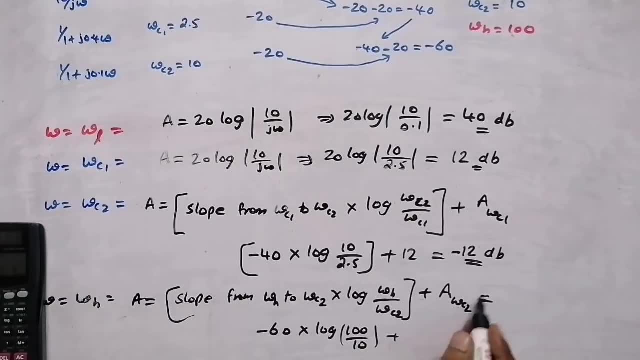 be multiplied by log of omega higher. Omega higher, it is 100.. Divided by omega c2.. Omega c2, it is 10.. That should be added with the previous value, That is minus 12.. What we will get, We will get. 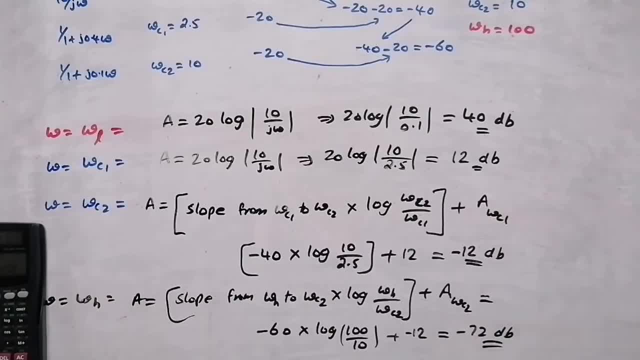 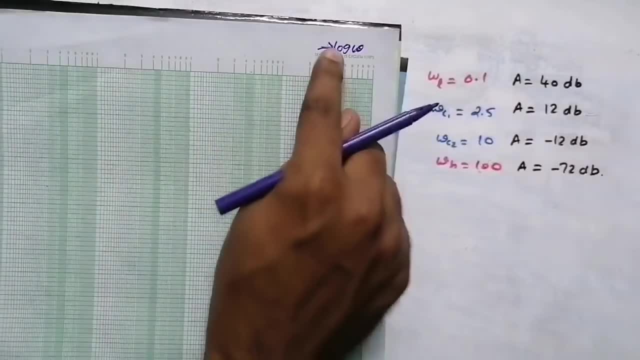 the answer as minus 72 dB. So these are our magnitudes. So with this frequency and magnitude we are going to draw the magnitude plotting semi-log graph. As we know our x-axis it is magnitude. That is log value, log of frequency. So wherever you can see 1, you can see 1 here. 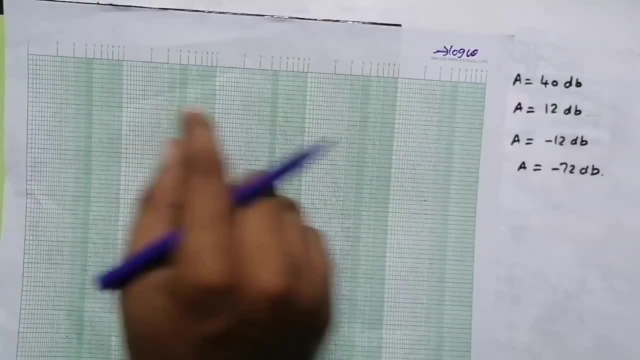 1 here, 1 here, 1,, 1, like that. All those 1, you need to replace with the powers of 10.. So the first value will be 0.1, because I selected my log frequency as 0.1.. Then the next one. 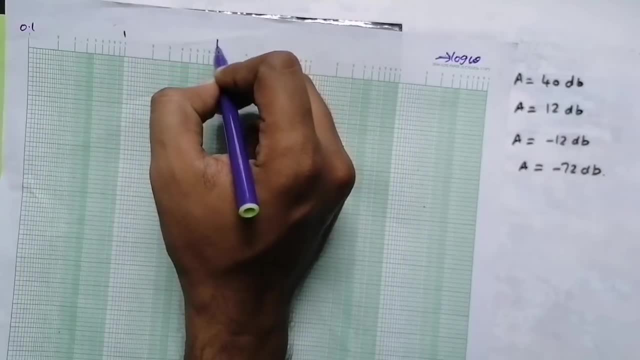 it is 10 raised to 0.. That is 1.. The next one, 10 raised to 1.. That is 10.. Then this one, 10 raised to 2.. It is 100.. Then this one, 10 raised to 3.. It is 1000.. Then it is 10 raised to 4,. 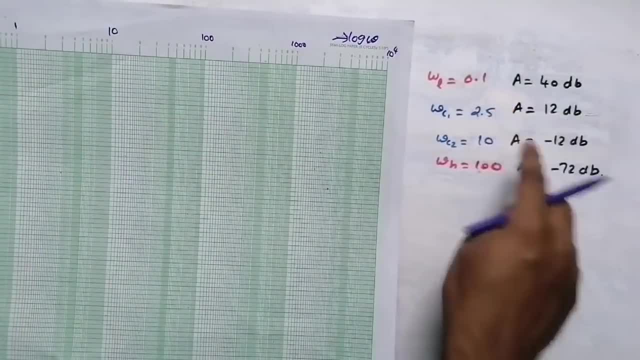 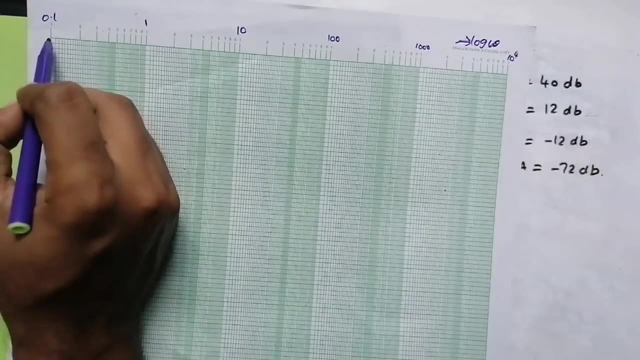 the last value. Now I need to draw the magnitude. So my y-axis, Y-axis, will be magnitude My highest plus 40. So I am going to write: I can take 50 or 40 here, I will take 40, okay. After 5 lines. 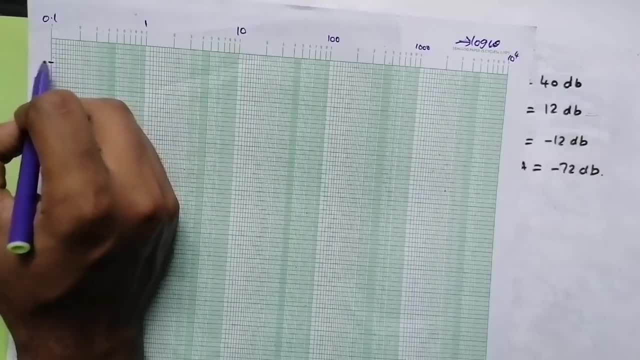 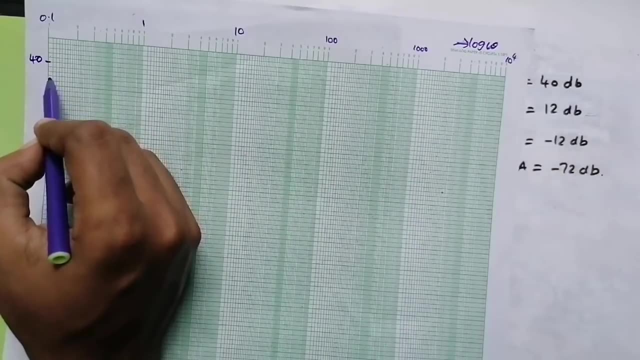 1,. after 5 small boxes: 1,, 2,, 3,, 4, 5.. Here I am going to write: plus 40 dB. That is my highest magnitude in this section. Then again, after 5 boxes: 1,, 2,, 3,, 4, 5, my next magnitude Then. 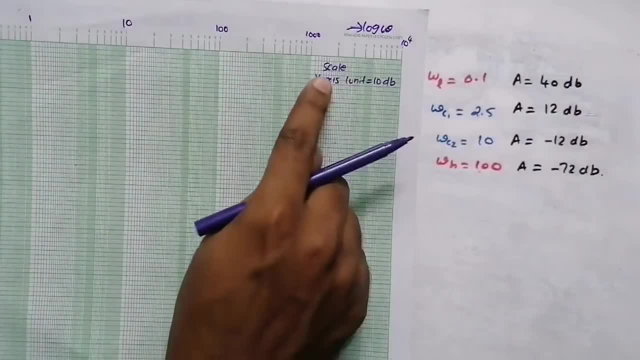 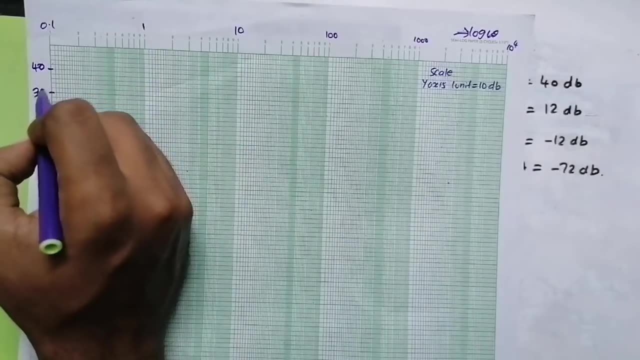 again after 5 boxes. my next magnitude, like that you need to plot. I am going to take my scale of y-axis as 1 unit. it is 10 dB. 1 unit is after a 5 box gap. okay, So 40,. this one is 40. Then 30,. 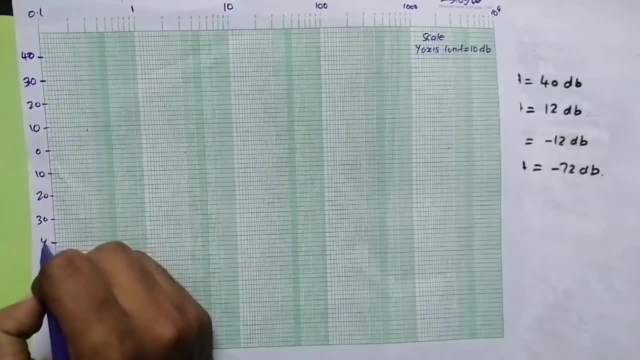 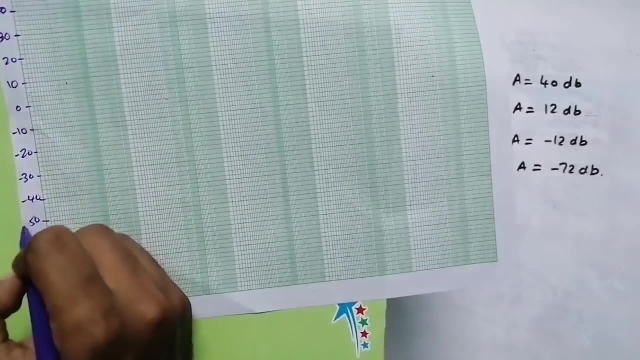 10, 0,, 10,, 20,, 30,, 40,, 50, up to. I need to get up to minus 72. I need to get okay From here onwards, after 0, it is negative values, okay, Minus 10,, minus 20,, minus 30,, minus 40,, minus 50,, minus 60,. 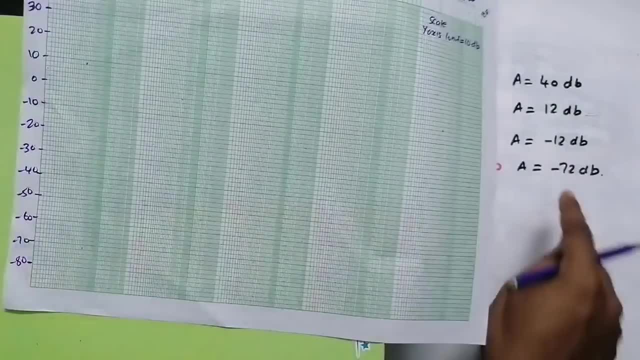 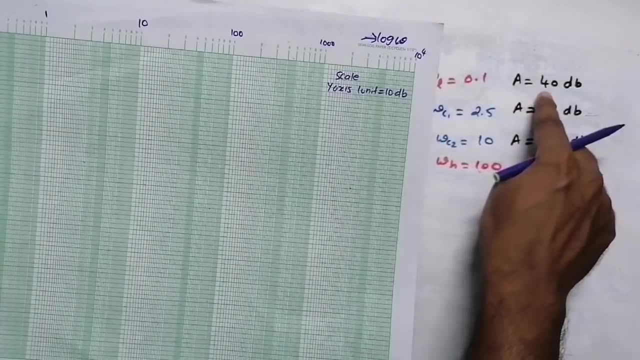 then minus 70,, minus 80. So I got minus 72 also. okay, So this is my magnitude plot. Now I need to plot this point in the graph. So, first of all, when omega dollar 0.1, my magnitude is 40. So 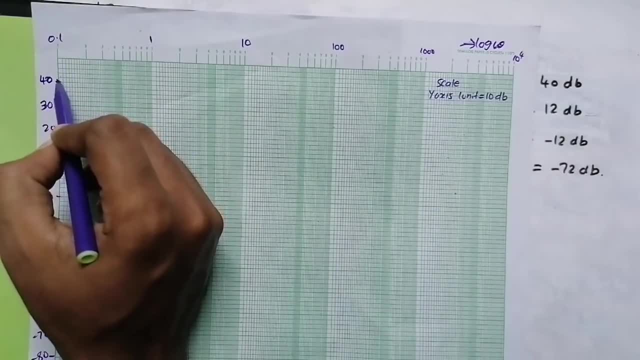 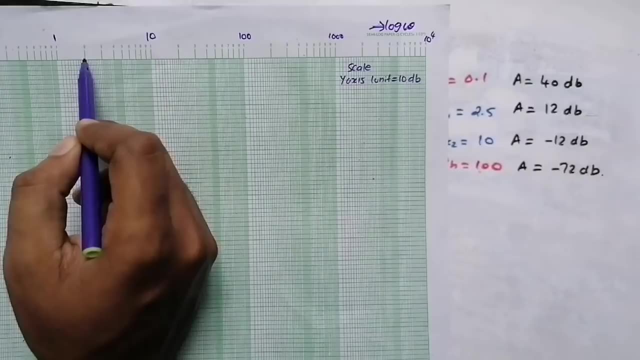 0.1, minus 0.1, 0.1 is here 0.1, my magnitude is 40. So this is my first point. Then the next point is 2.5, my magnitude is 12.. So where is 2.5?? This is 1,, this is 2, and this is 3.. So 2.5 is here. 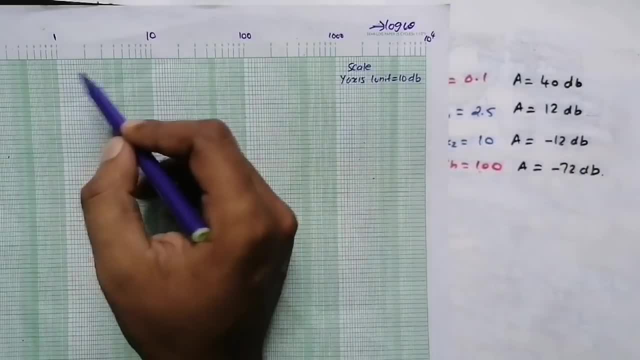 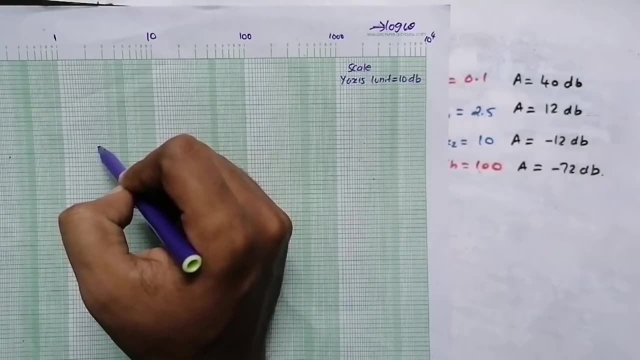 In between 2 and 3, it is 2.5.. At 2.5, my magnitude is 12.. So 2.5, my magnitude is 12.. So this is 10, then 12.. So here, approximately here. Then the next frequency, it is 10.. So 10.. At 10,. 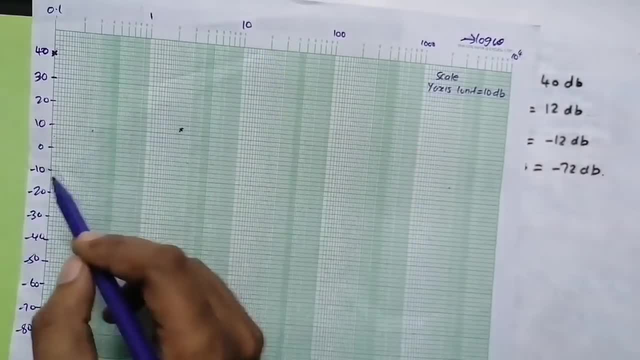 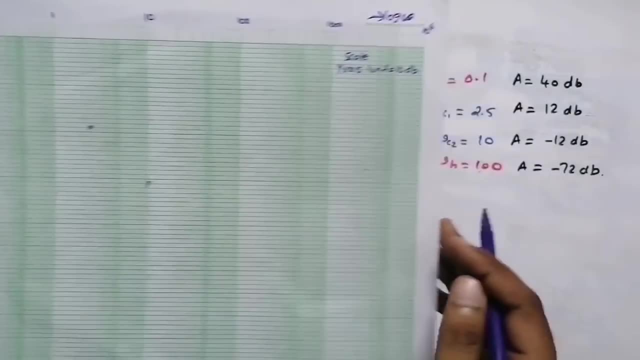 my magnitude is minus 12.. So 10,, my magnitude is minus 12.. This is minus 10, and this is minus 12.. 10,, my magnitude is minus 12.. Okay, then, higher, When omega h, higher at 100,, I will get minus 72. 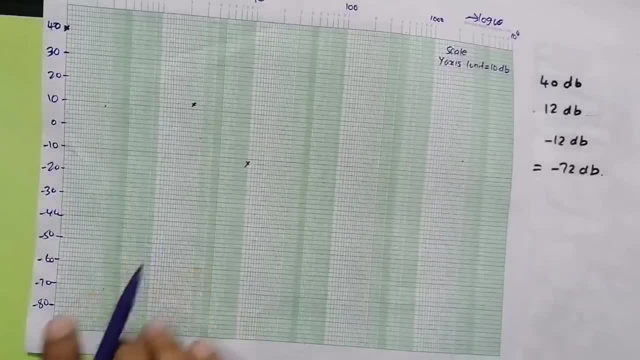 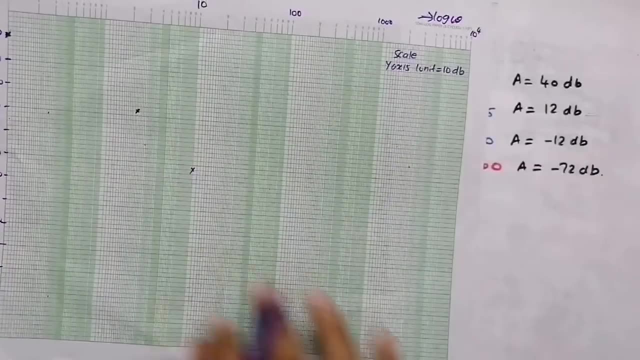 So this is 100.. At 100, I will get minus 72.. This is here. it is minus 70. So minus 72 will be here, So I will get it over here. So this is my point. Now join this using scale For magnitude plot. 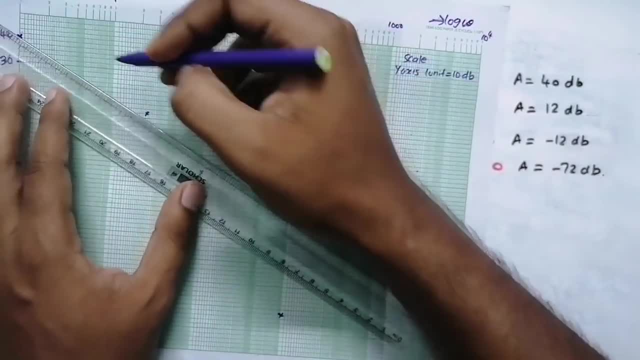 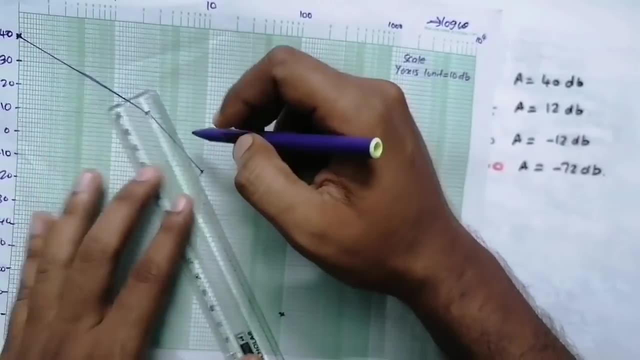 you need to use scale. Join this point using our scale. So from 40 to 12, first join the line, Then from there join to the second point, Then from there join to the third point. So this will be our magnitude plot graph. Okay, from the table. 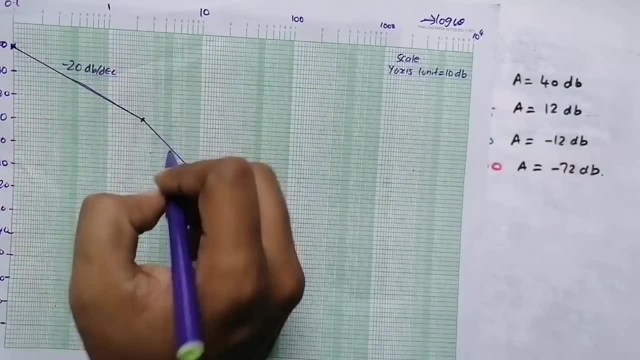 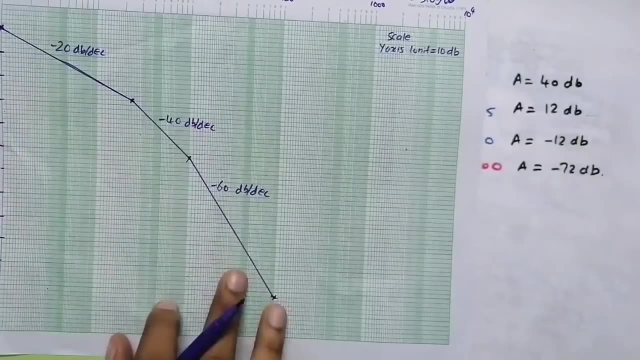 we got the first change in slope. it is minus 20 dB per decade. Then after that, the change in slope is minus 40 dB per decade, And after that the change in slope is minus 60 dB per decade. So this is the magnitude plot. Now, after plotting the magnitude plot, we need to draw the phase. 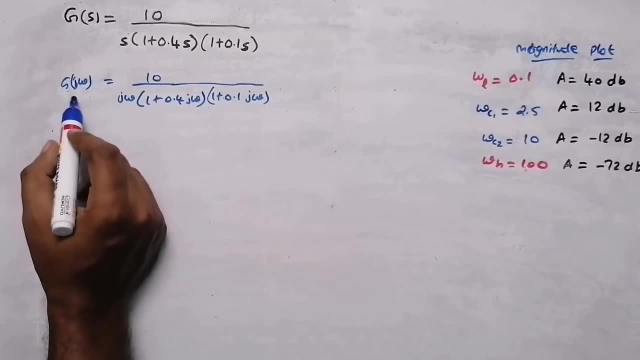 angle plot. For that we need to find the phase angle. Okay, phase angle of g, of j, omega, that is 5, phase angle. So there are three terms. These are first term, second term, third term. Okay, 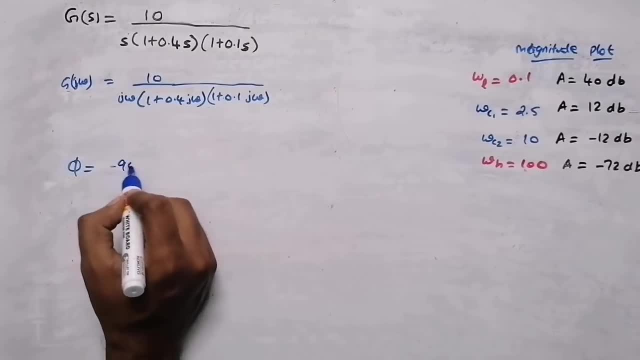 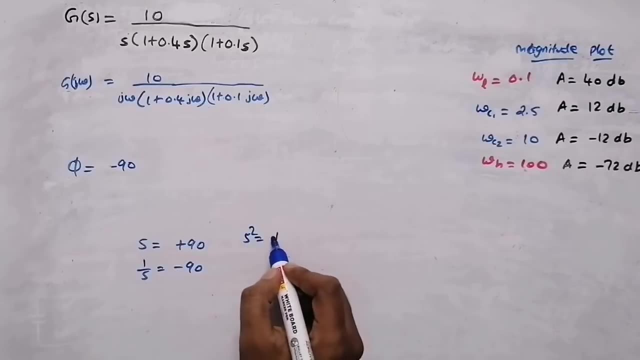 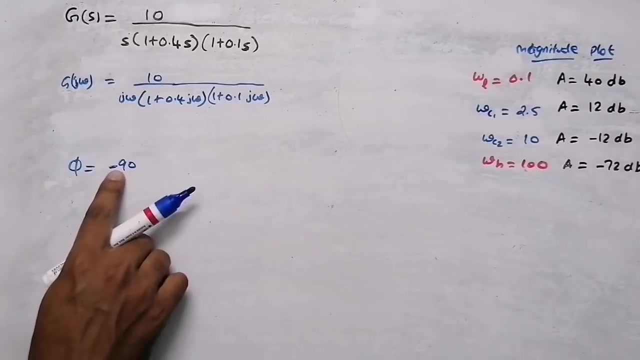 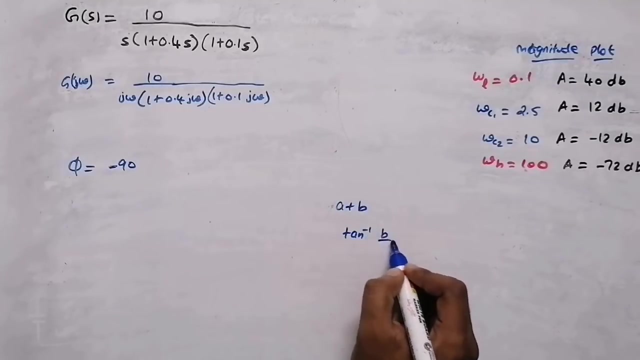 then this is 1 by A here. First term is- this is the third term- Jegune was거� 90 degrees below the wentoshkan in the denominator. So and a is in the denominator. So if it is in the denominator, the angle would be minus 90, if s is in the denominator, the angle will be plus 90.. If s is the denominator, the angle will be minus 90. If s is in the denominator, the angle will be plus 90.. If square is in the Numerator triangle will be plus 180.. If square is the denominator, then that would be minus one. order Like that Here. our first time isn't a denominator, So we want minus 90.. Now the second time. second time it is of the form a plus b And how to find the angle. we founded tan, inverse B by B. so this is our day and this is our baby. Then we need to find tangles. 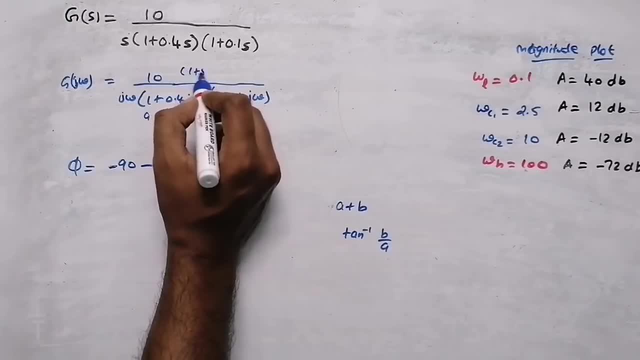 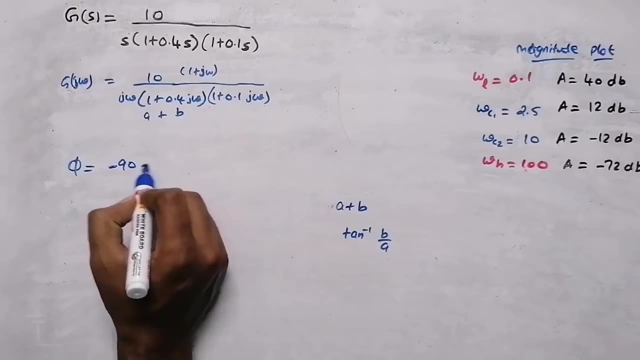 the second time in the denominator. we need to put minus if the term was here. if the term was here, then we will put plus. if the term was in the numerator, we will put plus sign. if the term is in the denominator, we will put minus sign. so here the term is in the denominator now. tan inverse b. 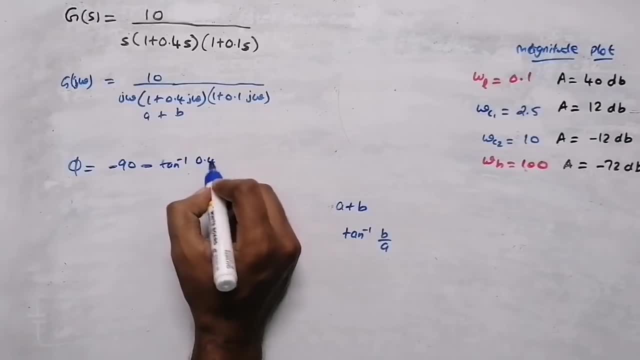 by a. what is our b? 0.4 omega. so 0.4 omega. divided by a, it is 1. so 0.4 omega by 1, it will be 0.4 omega itself. you do not do not want to take the j time. okay, only the omega values. now the next. 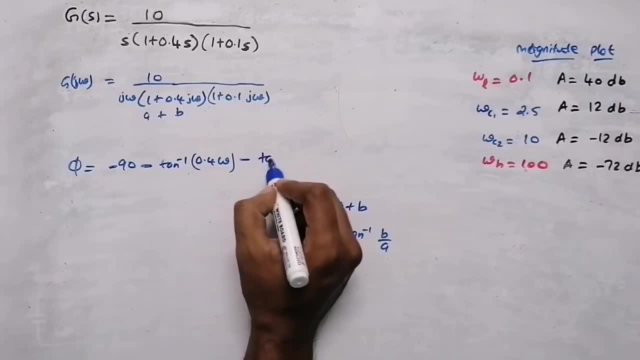 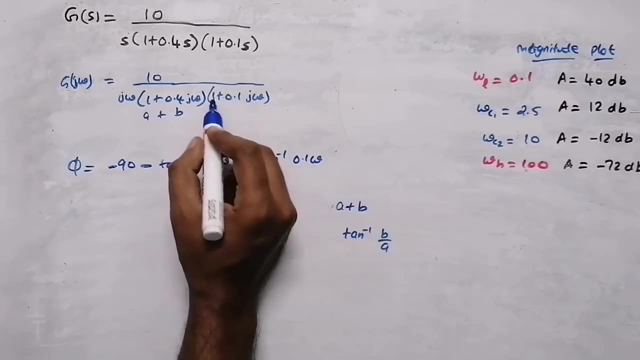 time, next time also, it is in the denominator, so the sign will be minus. then tan inverse b by a, b is 0.1. do not take j, only omega you want to take. so 0.1 omega, 0.1 omega divided by 1, so you get. 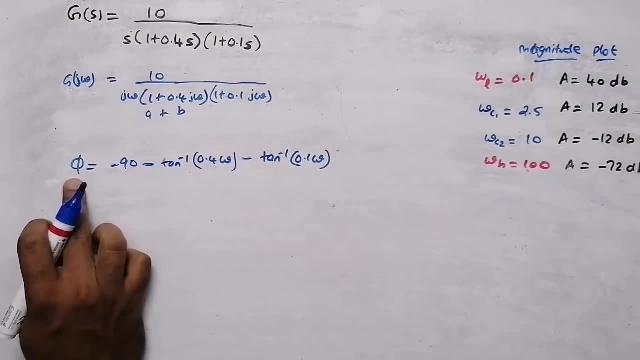 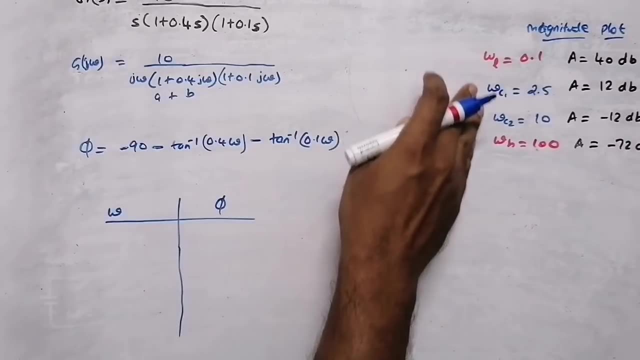 like this. so this is the equation for finding the face angle. now we need to draw a table which consists of omega and 5. we need to draw a table. we should take all the values that we took for writing the magnitude plot. all the values should be there. that is, we should take 0.1, we should take. 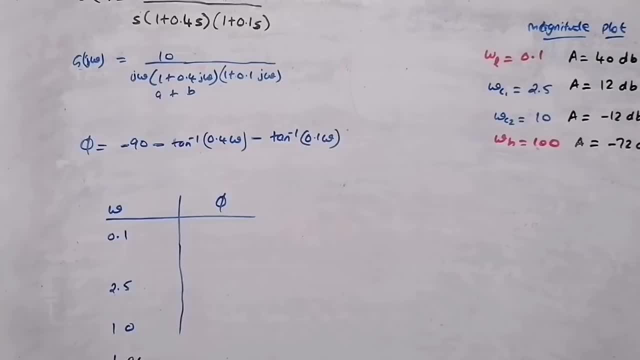 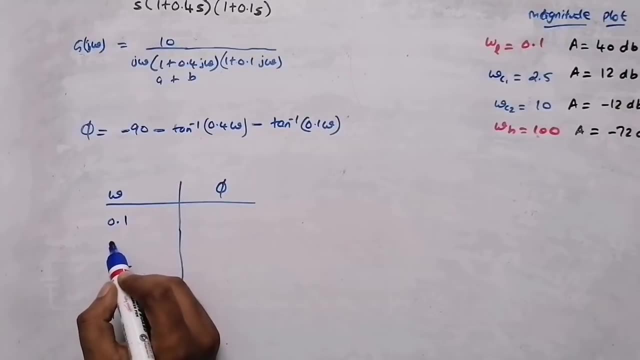 2.5, we should take 10, we should take 100, all those values we need to take. other than that, we should take some more values to make the answer more precise. okay, so 0.1 i do, then the next time i will take 0.5. then 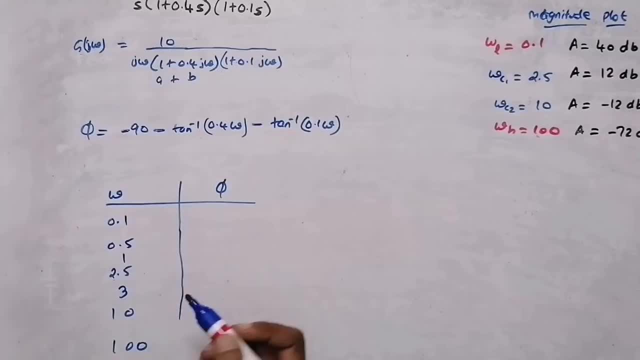 i will take 1, then i will take 3, any values you can take in between that, any values you can take, then i will take 20, like that. okay, now for corresponding omegas. i need to find the angle by using calculator. so you can use calculator for that. you need to type this equation and find the. 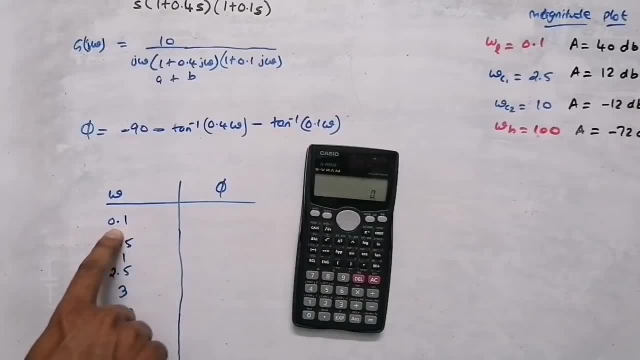 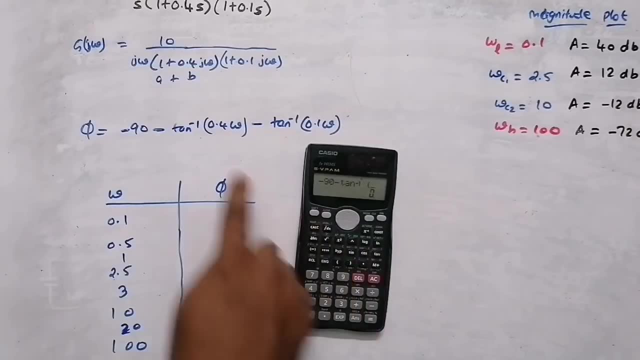 answer corresponding for that i will show you. for 1, 0.1, i will show you how to find the angle remaining. you need to find: okay, so 0.2, 0.1, that is minus 90 minus tan, inverse 0.4 into omega. instead of omega i need to write 0.1, so 0.4. 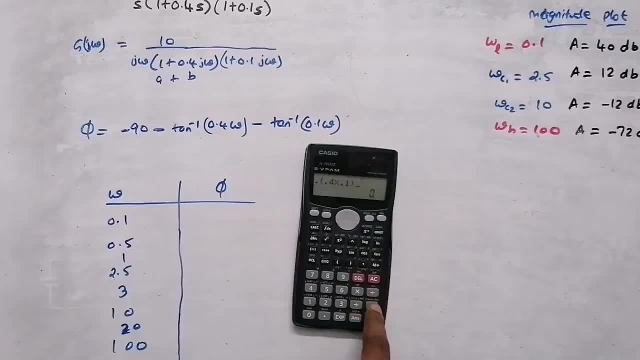 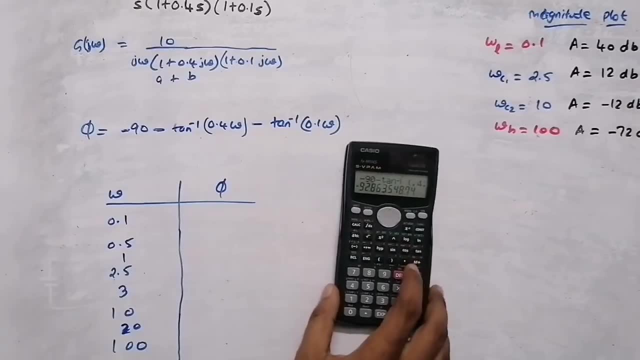 into instead of omega. i am writing 0.1. okay, then minus tan inverse, then 0.1 into omega instead of omega. i need to take 0.1, then i will get the answer as minus 92.86. that is approximately i can take it. 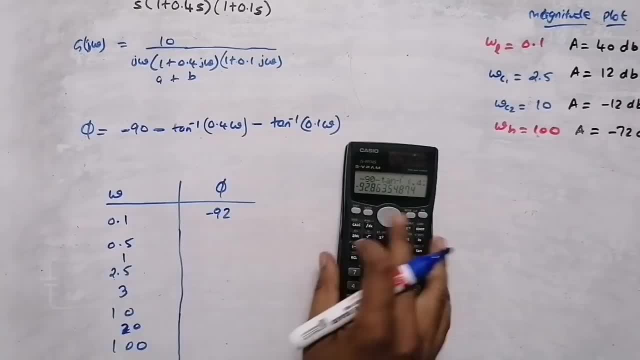 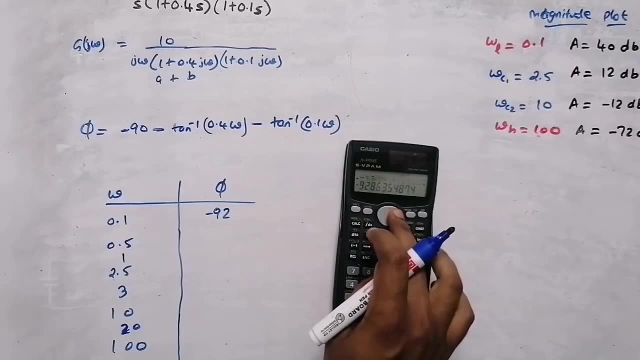 as minus 92 itself. then for 0.5. okay, substitute here 0.5 instead of omega. you need to substitute 0.5. so when we substitute 0.5 here, you will get the answer minus 104. okay, now, like that. do the remaining angles? find the angles for. 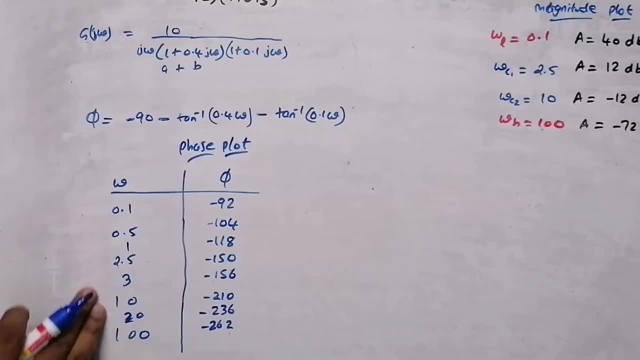 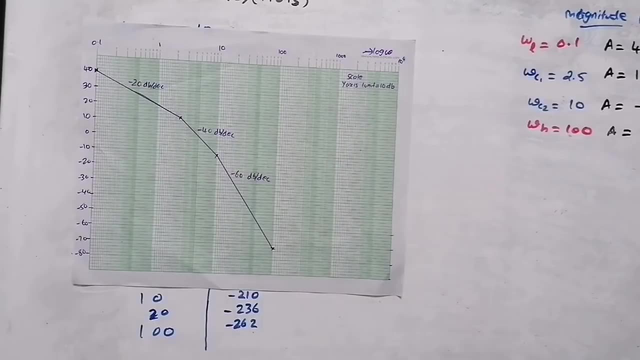 remaining omegas. so after substituting the values for omega in this equation, we will get the angles like this: now we need to plot this angle in the graph sheet. now, for drawing the face angle plot in the graph sheet, we need to take this axis. okay, here we look. magnitude plot axis- here we 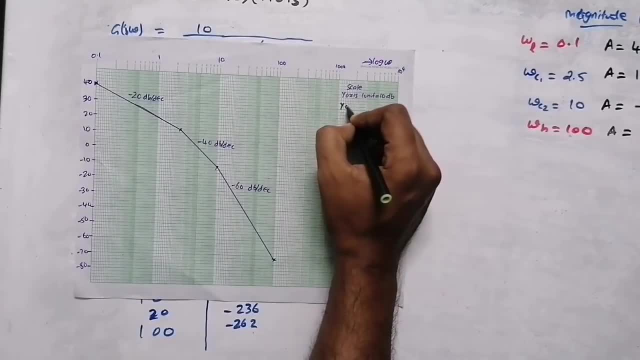 need to take the angular plot axis, so y axis. one unit will be. i'm going to take it as 20 degree, okay, so the highest angle it is 262.. so i'm going to eliminate both angles and we will理 Пn of y and mean estimator. 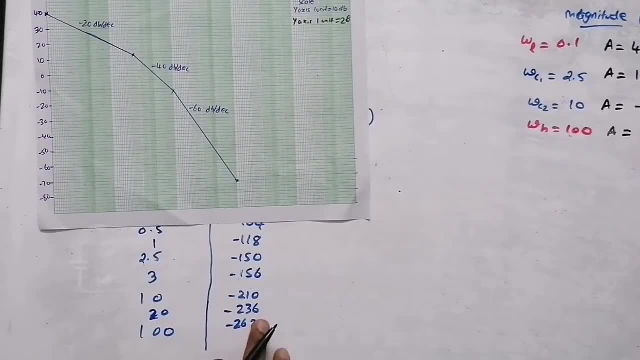 So Y-axis will be, 1, unit will be. I'm going to take it as 20 degree. okay, so the highest angle it is 262.. so i'm going to eliminate that because it is a high value. i can take 236 as the highest value. 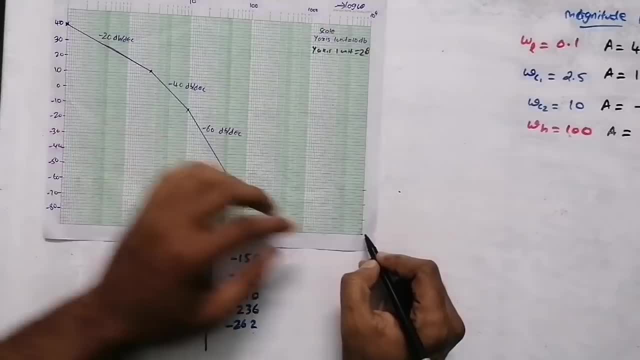 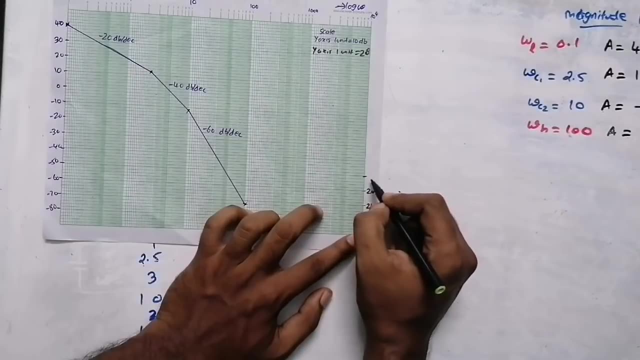 then the highest value i need to mark here, so 236, so i'm going to mark it as 240. okay, then at the gap it will be 220, 210, then 200, then after a five degree gap it will be 180, like that we need. 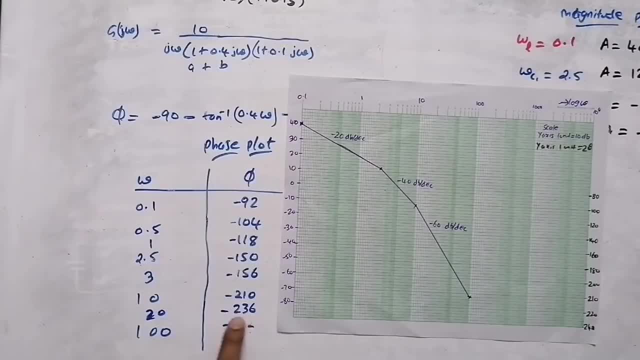 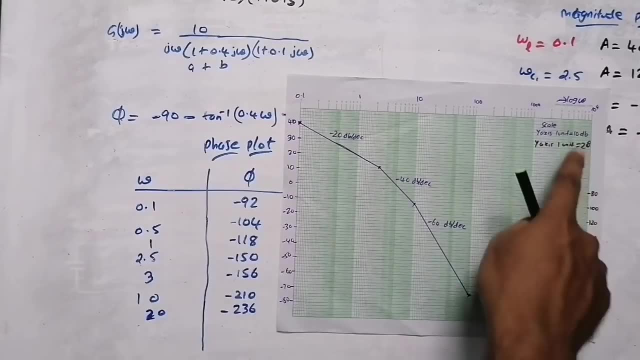 to move up. so the highest value, i took it as 236. i eliminated this thing because already there are. the graph is very big, so i generated the highest value and this minus 236. so i took minus 240. then, at a gap of 20 degree, 220, 210, 200, 180, up to 80. so here it is up to 92, so up to 88 the maximum. 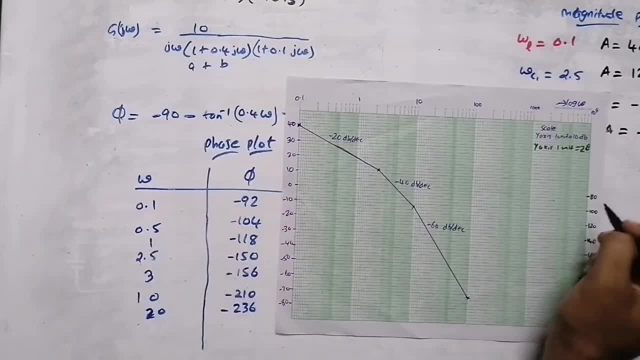 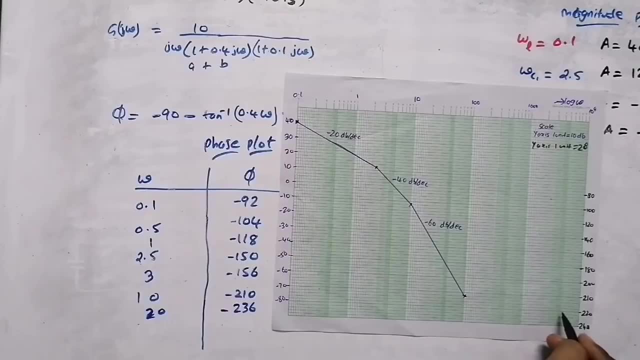 value and minimum value. you need to look. so 240 and 80- all these are negative values. okay, negative values. since these are negative values, i started highest value from here. if the angles are positive, i need to start zero here: 10, 20, 30, 40, 60, like that. i need to go understood if i'm getting positive. 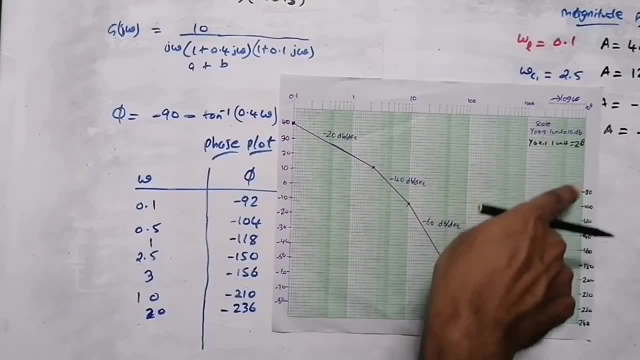 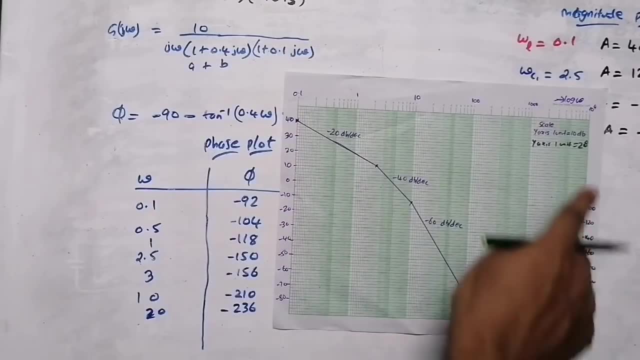 values. i need to start zero here. if i'm getting negative value, i need to start zero from the top to bottom. i think you understood. okay, if i get negative values, you need to come down. i need to start from highest to lowest. i'm getting positive values- and to start from lowest to highest. 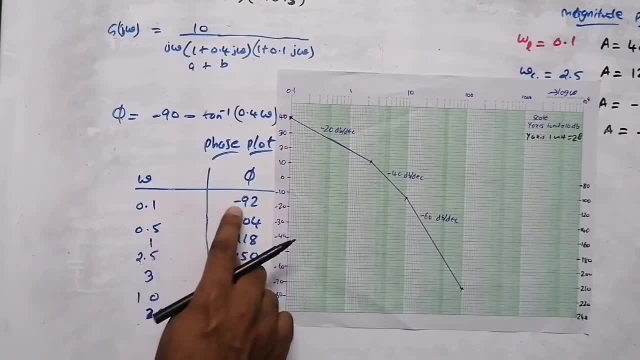 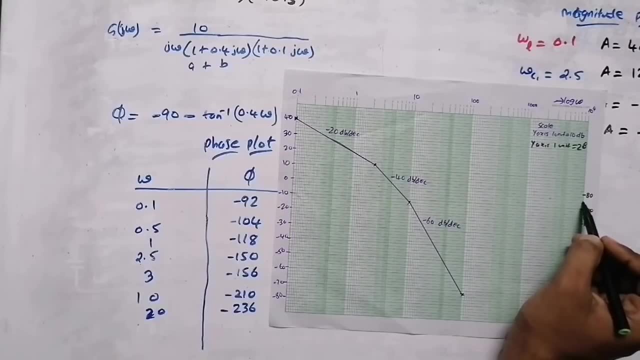 that is the only difference. okay now, at omega equal to 0.1, my angle is minus 92.. so omega is 0.1, my angle will be 92.. so this is 80 and this is 100. in between that it is 92. so this is 90- 92. 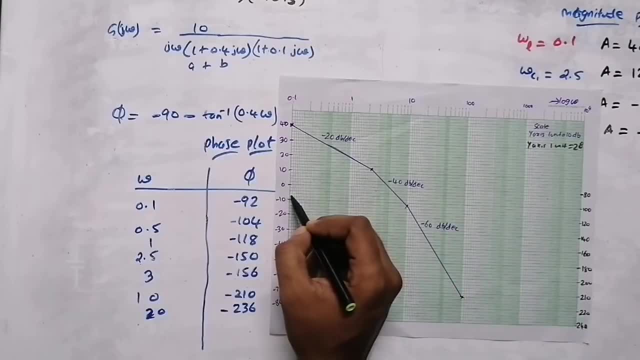 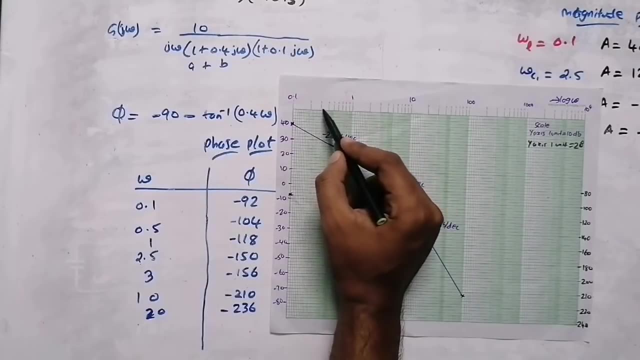 will be approximately here. so approximately here at omega equal to 0.1. i will get the angle here now. omega equal to 0.5. it is minus 104, 0.5. 0.5 is here: 0.1, 0.2, 0.3, 0.4, 0.5. so at 0.5. 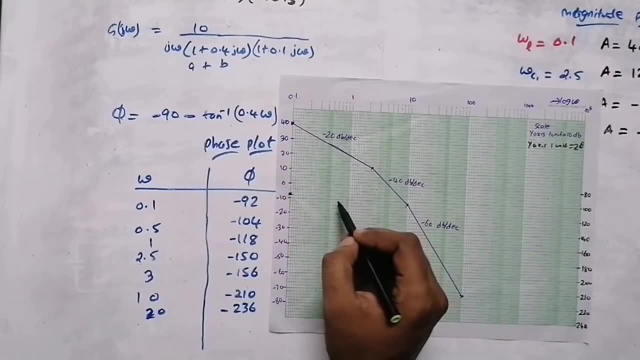 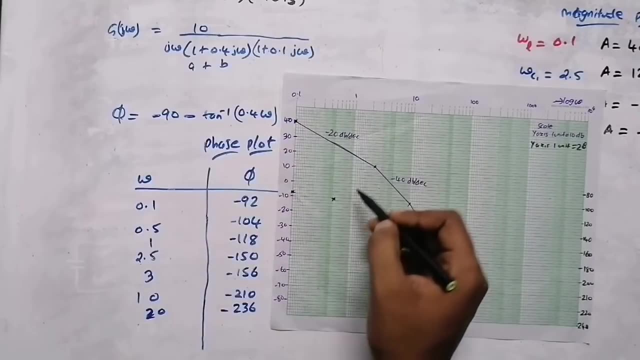 my angle is 104, so it is approximately here at 0.5. okay, now 1 at 1. my angle, face angle- is minus 119.. 1 is here and my angle is 118. 120 is here, so 180 will be approximately here. you can use a scale for plotting the points, okay. 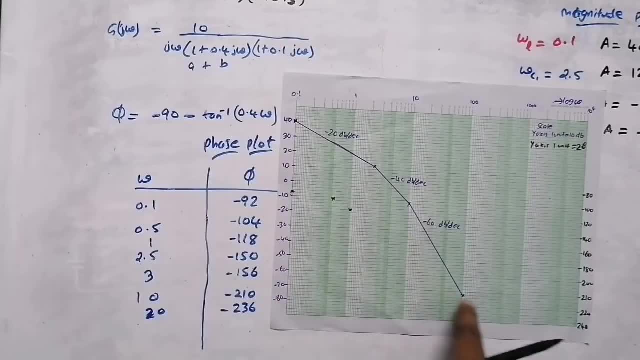 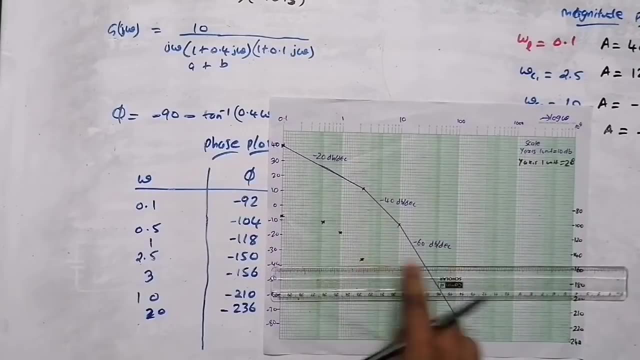 here, then 2.5. my angle is minus 150, like that plot all the points. now at 3 my angle is minus 156.. so 3 is here. 1, 2, 3. my angle is 156, 150 is here, so 156 will. 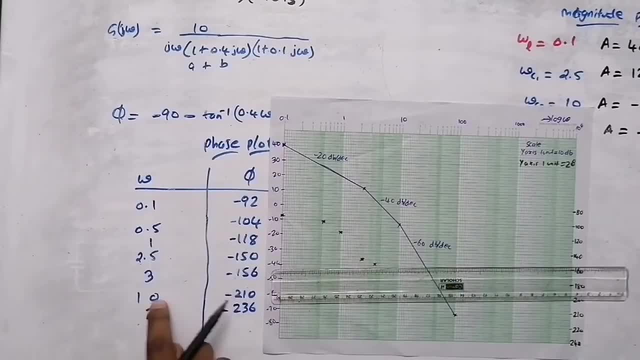 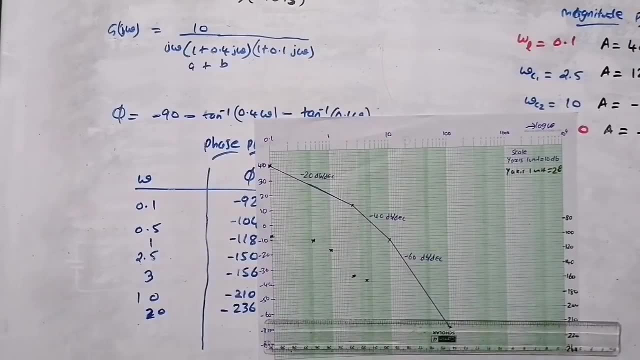 be approximately here. so at 3 my angle will be 156, then at 10 my angle will be minus 220, 210. at 10: 210, okay, 220. oh my god, i made a mistake here. i made a small mistake here. after 200 my angle the gap is 20 degree. i got 210 here, so 220 i need to. 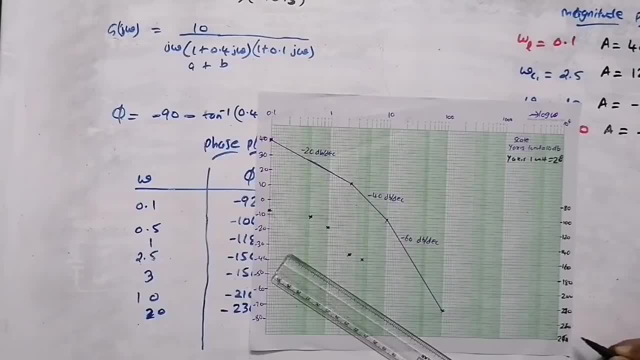 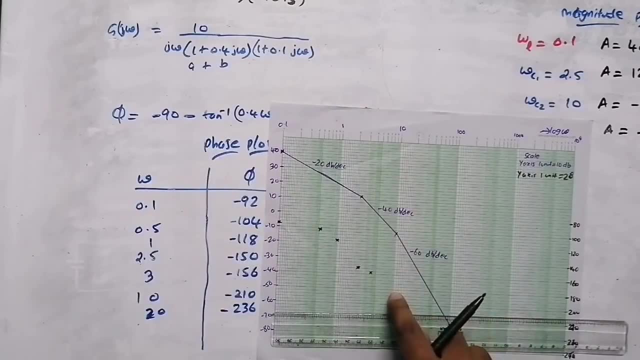 plot: 200, 220, 240 and the final value will be 260.. okay, at 3 at 10, i am getting minus 210. at 10, i am getting minus 210. my 210 will be approximately here at 10.. so you can use scale and mark the. 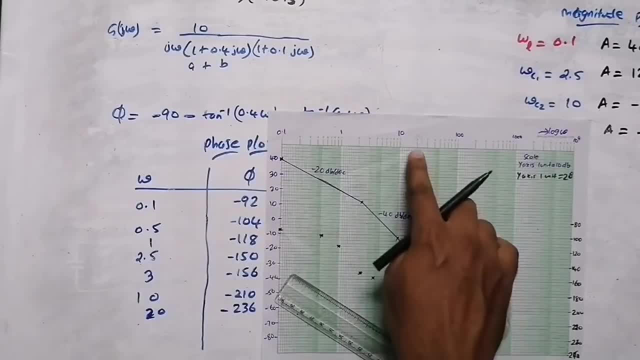 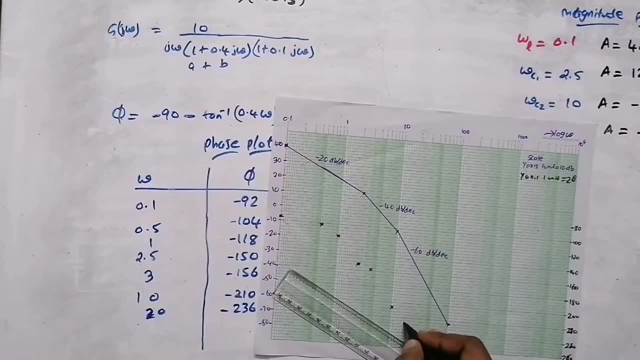 point. then at 20 i am getting minus 236.. so 20, 10 is here. so 20 is here, 20, i am getting 236.. so this is 220 and 240. it would be approximately here 236, 20.. okay, now for drawing the phase plot. 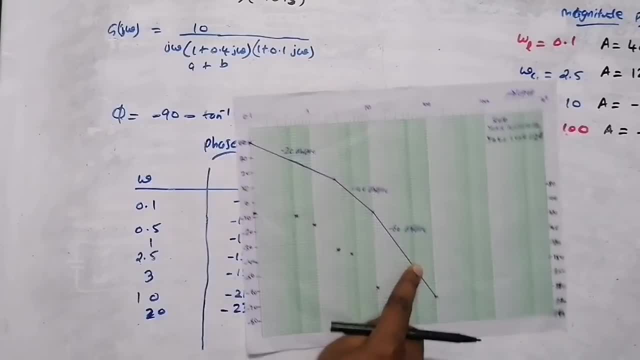 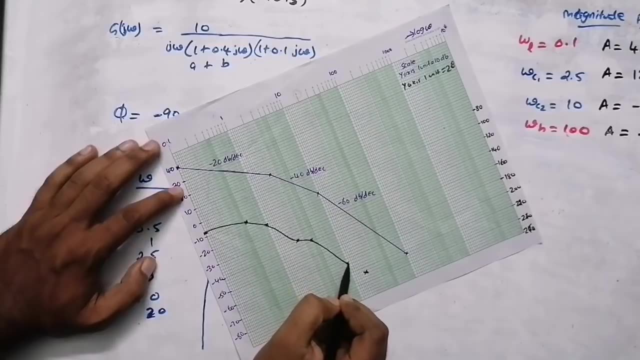 you can use free hand. for drawing magnitude plot, you need to use scale, but for drawing phase plot, you can simply use your free hand and join the points like this: see: join the points like this, so this will be our phase plot. so thus we get the magnitude plot and this is our phase plot from. 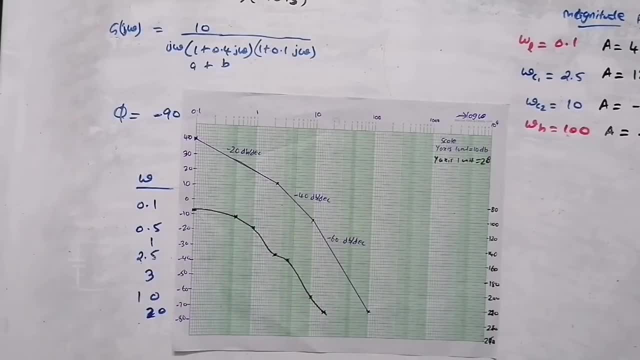 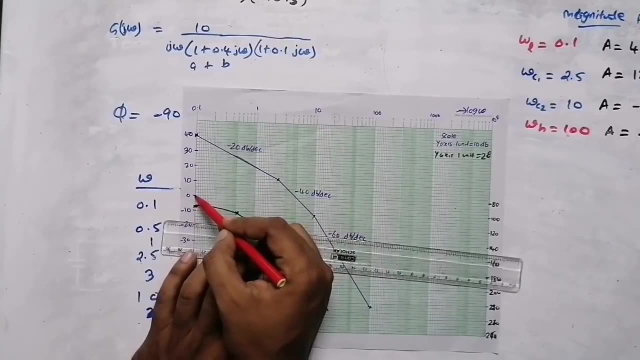 this we can find the gain cross of frequency and phase cross of frequency. for finding gain, cross of frequency. this is our gain, magnitude is our gain. for finding gain, cross our frequency. first of all, check our zero. where is our zero here? from zero, draw a straight line. from zero, draw a straight line like this. so this: 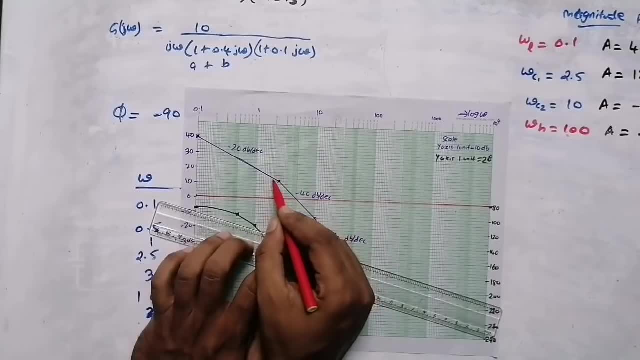 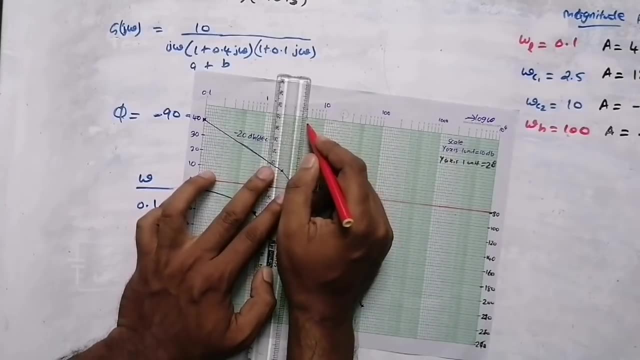 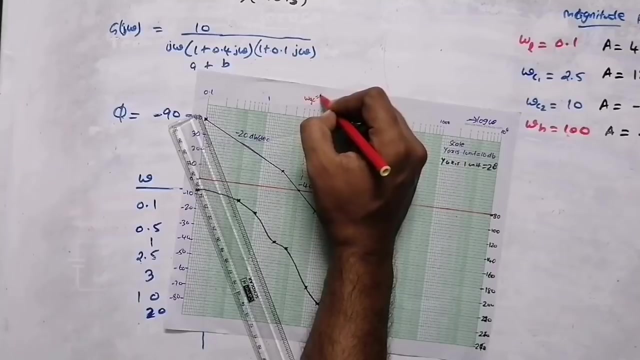 is a straight line from zero, the point. the magnitude plot will touch the zero at a point here it is touching. check that frequency, check that frequency. that frequency, it is five radian per second. it is one, two, three, four and five. so five is our gain. crossover frequency. 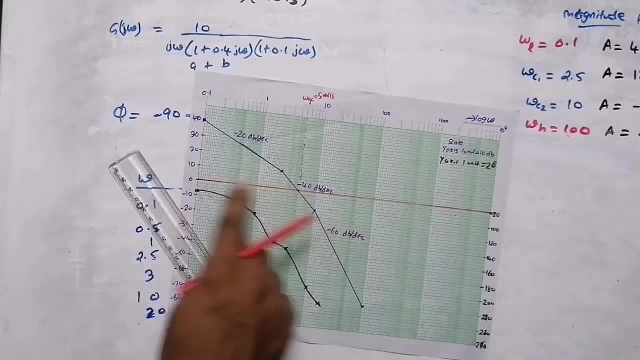 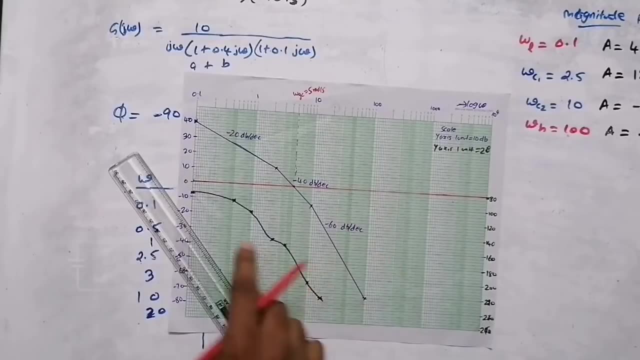 five radian per second- that is our magnitude- will cross zero db at a point. that point is our gain. crossover frequency: i hope i made it clear to you now phase crossover frequency. for finding phase crossover frequency, take minus 180 degree. so this is minus 180. you can see here: minus 180. 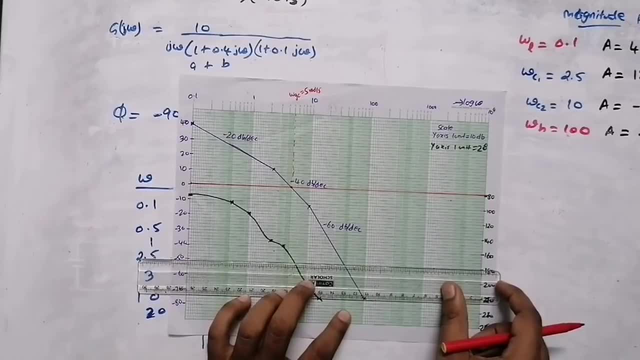 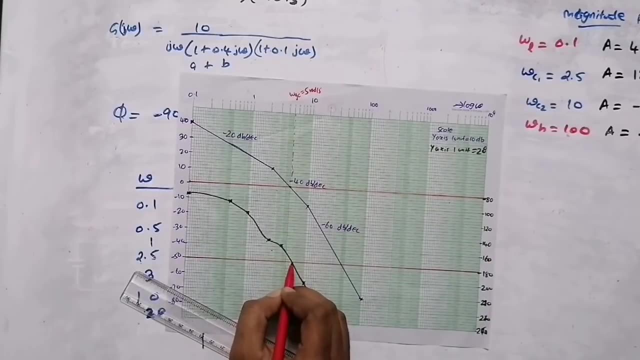 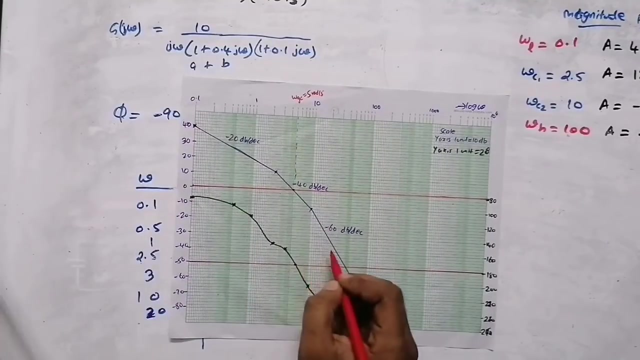 draw a straight line from minus 180. so from minus 180, draw a straight line. okay, now the phase plot will touch minus 180 at a point here you can see it is touching at this point. so our phase plot will touch the minus 180 degree line at a point plot. check that point, that point. 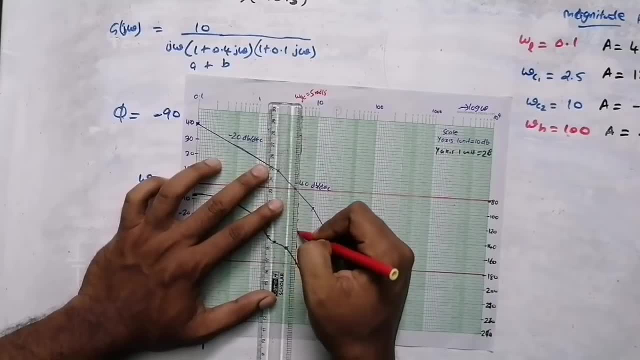 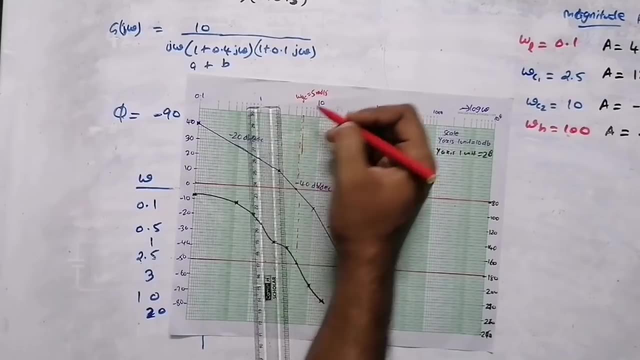 that point is nearly close to five, so we can take it as five point two or five point three, or we can take it as five also. okay, so i'm taking it is between five and six, so i'm taking it as five point five. radian per second. that is my omega pc phase cos of frequency. this was my gain, cos. 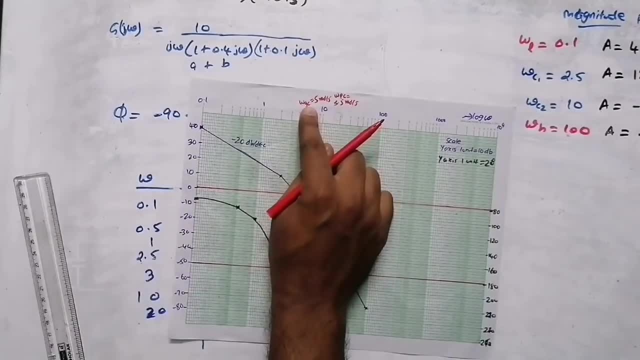 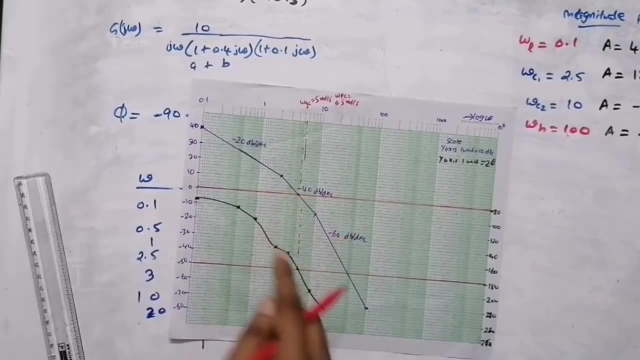 of frequency and this is my phase cos of frequency. for getting gain cos of frequency, draw a line from minus 180 degree where our gain plot is touching. so here it is touching. for getting phase cos of frequency, draw a line from minus 180 degree. then check our phase plot where it is touching. here it. 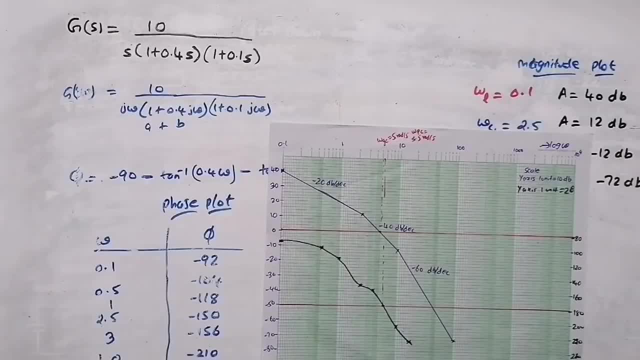 is touching that frequency. it is phase cos of frequency. if you have any doubts, just mention it in the comment section.